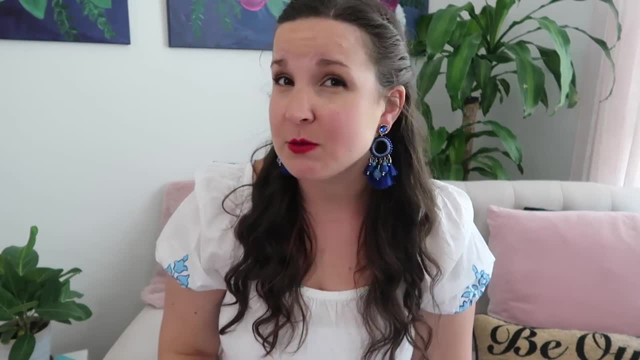 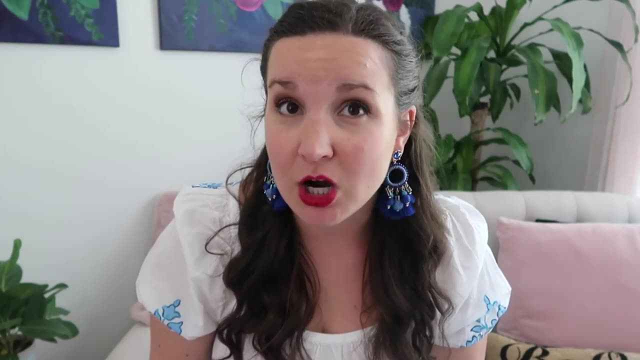 things about teaching that you can't learn. So in this video I'm going to give you a couple of tips for new music teachers, so that you will feel at least a little more prepared for what is coming next. Now, if you are a new music teacher, I will mention I have a free music teacher course. It's 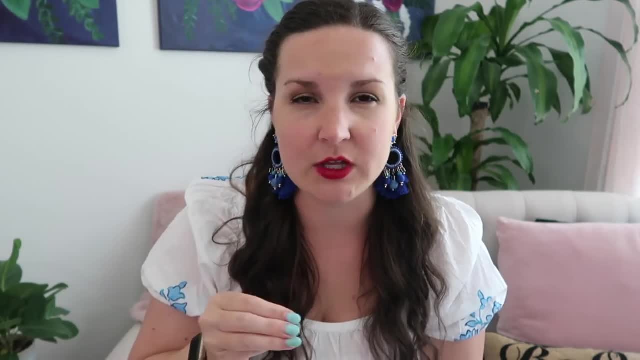 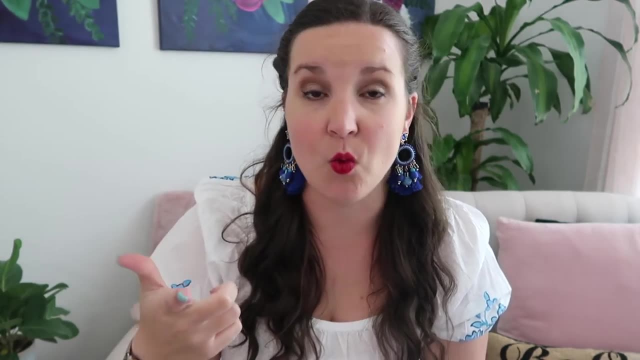 like a week long, And every day I send you like a really short video, really quick, with some links and different things to help you out. that covers things like classroom management And we cover things like what are you actually going to teach and how to teach rhythm and how to teach melody. 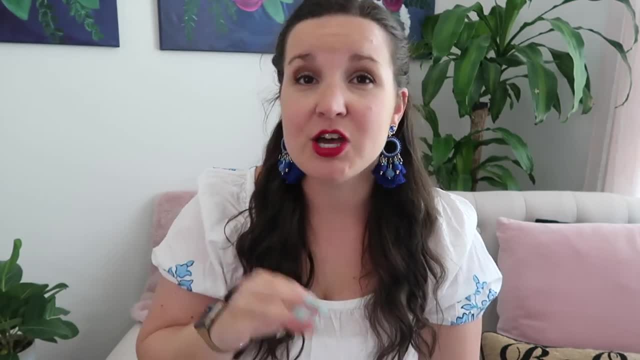 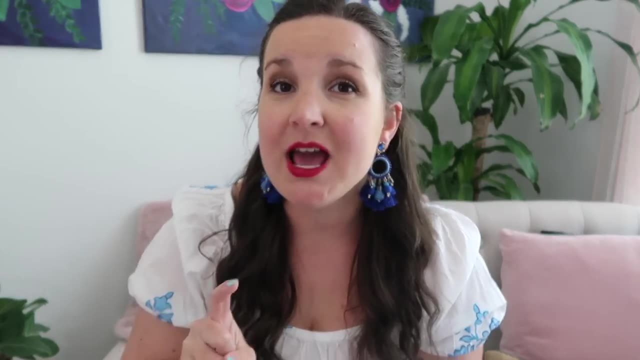 and all of those really helpful things. So I will link that down below. You can sign up down below. It's totally free And, yeah, let's get started. All right. So there's a couple of different tips I have here, but number one is the most important And that is number one. 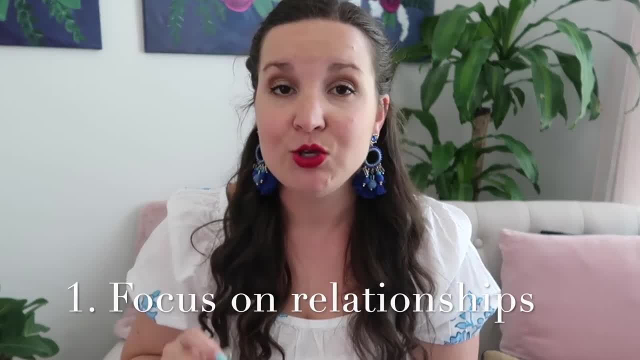 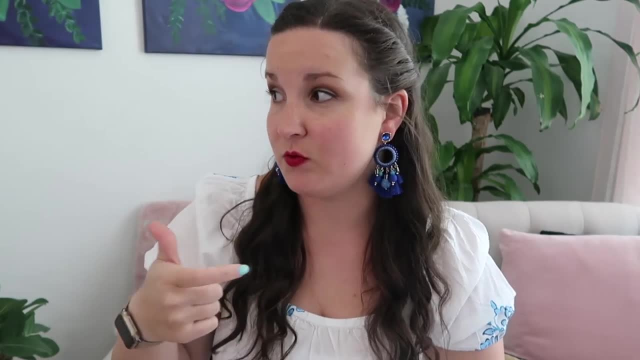 focus on the relationships When it comes to teaching children. you need to form a relationship with the child so that they will want to learn, so that they will feel like you know, an actual human being, And so that they will want to, you know, do things for you. Having relationships. 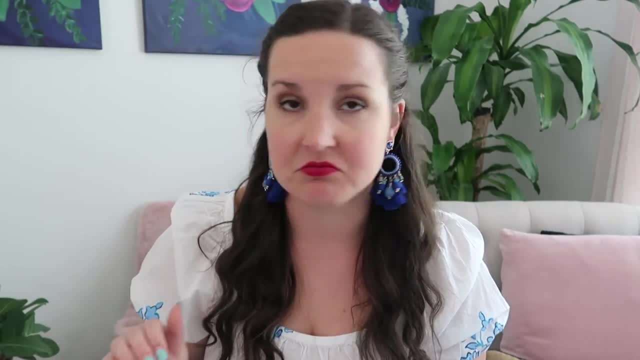 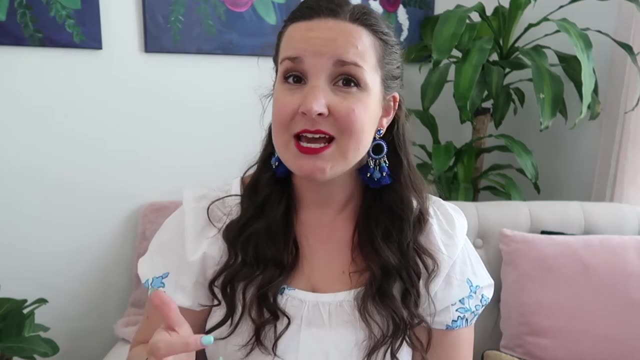 with students is the number one most important thing in teaching ever at all. I'm sure you can think of maybe a teacher that you really liked and a teacher that you really didn't like, And probably the main thing between them is that the teacher you liked 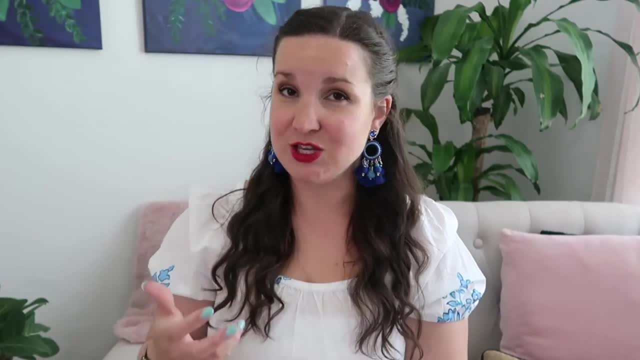 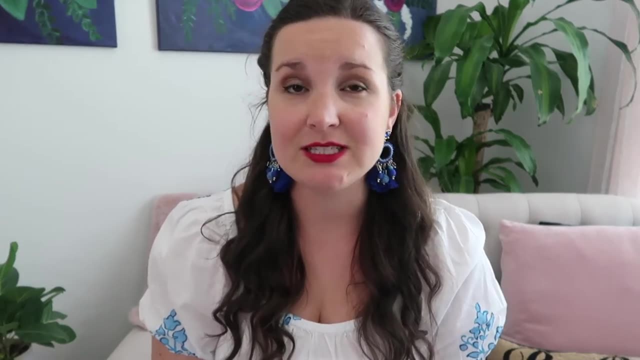 spent time to pay attention to you as a human being and actually treated you like a person and maybe even formed a relationship with you. It makes a huge difference- A couple of ways that you can focus on the relationships with your students when you have like a bajillion children. 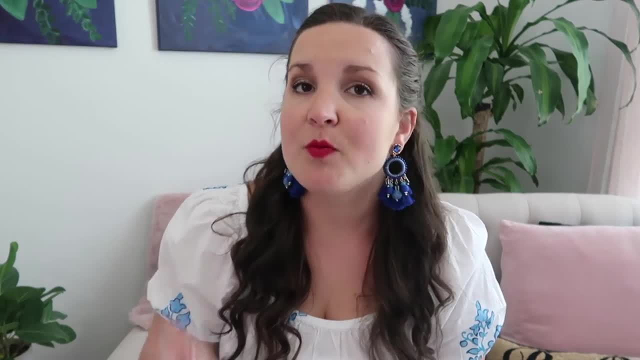 because, yeah, I've had years I had like 700 and I was like, oh my gosh, Number one is: use their names. Now again, 700 children, that's a lot of names. So my suggestion for this is to have a. 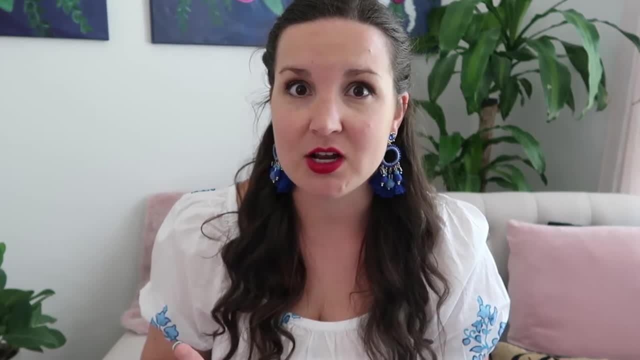 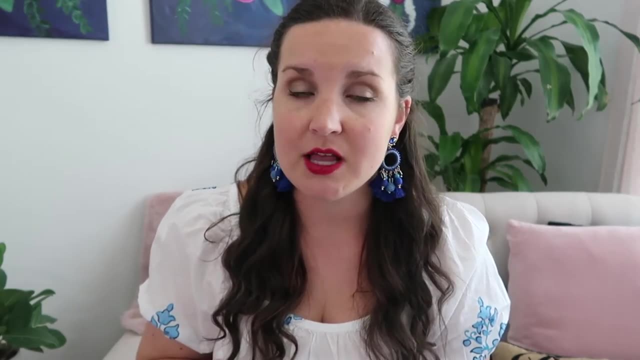 seating chart so that you can look at your seating chart and know like okay, that kid on the red dot is Johnny, because that's where Johnny's supposed to sit. Having a seating chart allows you to see like which kids are where and also allows you to try to cheat and figure out their names a lot. 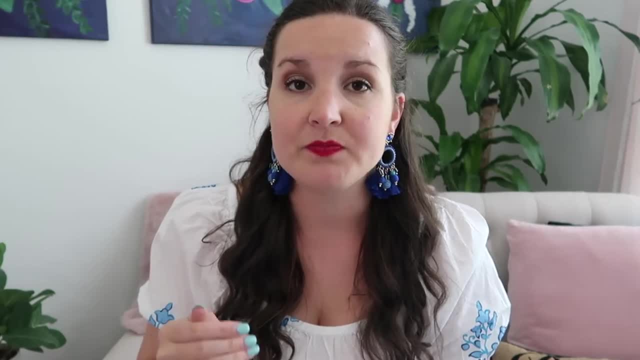 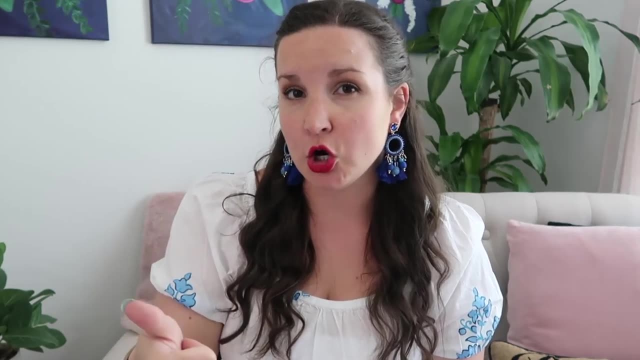 sooner. but use their names as often as you can, Even if you have to be like who knows X, Y and Z, Johnny, it's totally fine. But using their names makes the students feel like they are heard. It helps you to know that student better Cause when you know their name, like you know them. 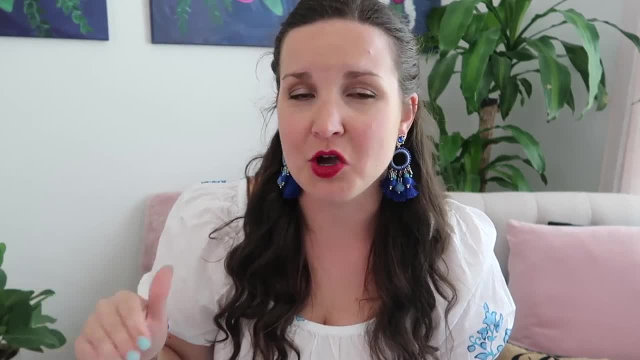 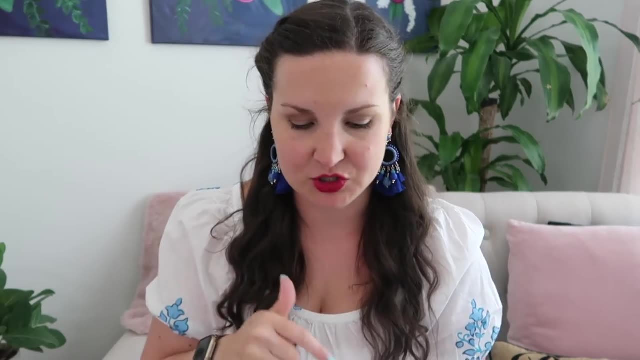 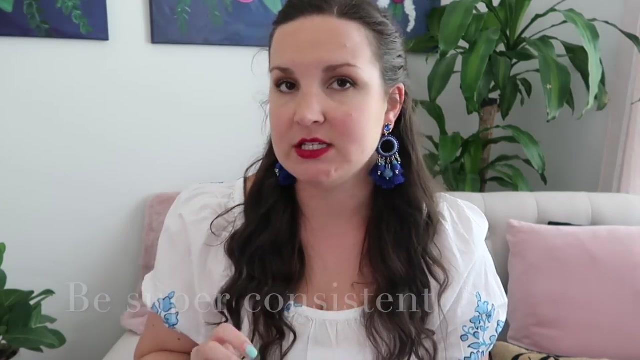 and in general, it just, it just makes everything go more smoothly. I promise, Try it. I will also link a video all about how to learn names quickly, as a music teacher down below to help with that, Along with learning their names, being super, super consistent is going to help. 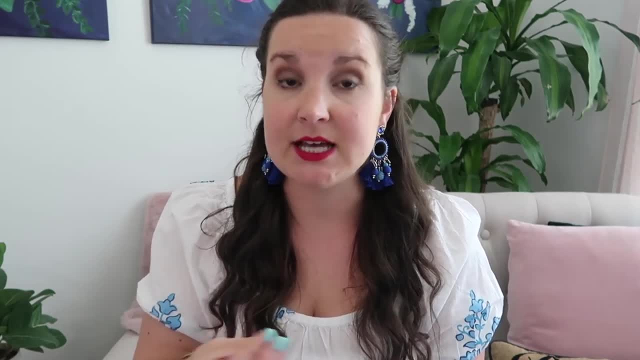 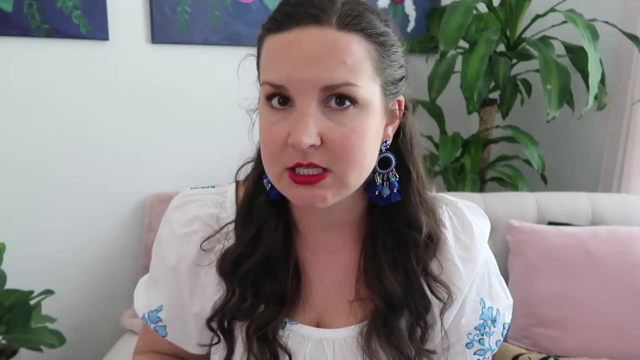 with the relationship building. This is especially important because, as music teachers, we typically see our kids like once a week, or I have my kids for a week at a time and then I don't see them for a month. So, whatever it is, you don't usually see them all day, every day like their classroom. 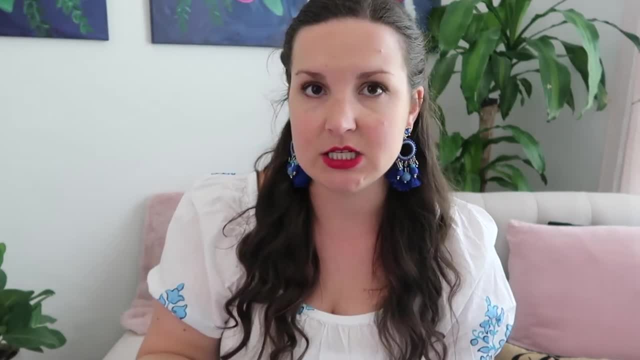 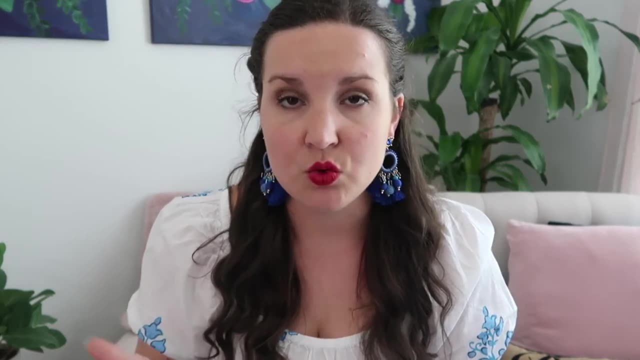 teacher And so if you can be very consistent in your demeanor, in your expectations and even a little bit in your class, then students will know what to do in your classroom And it kind of helps them to form the relationship with you. 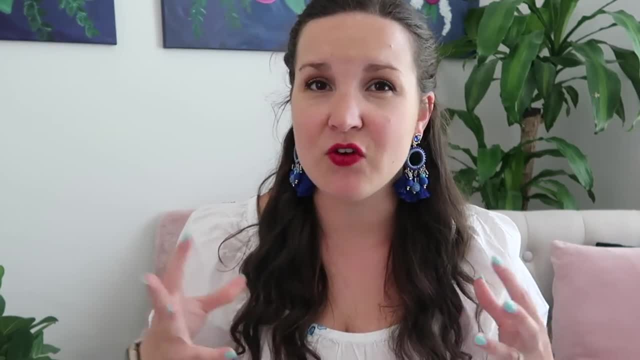 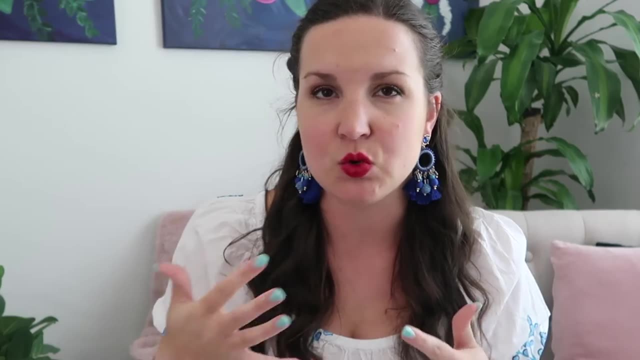 So I know that, regardless of what is going on, I have almost like a teacher persona. That's like what I do when I'm teaching, And it's not that I'm being fake, but it's just making sure that I'm being consistent and I'm showing up the way I want to show up. So when I see kids, 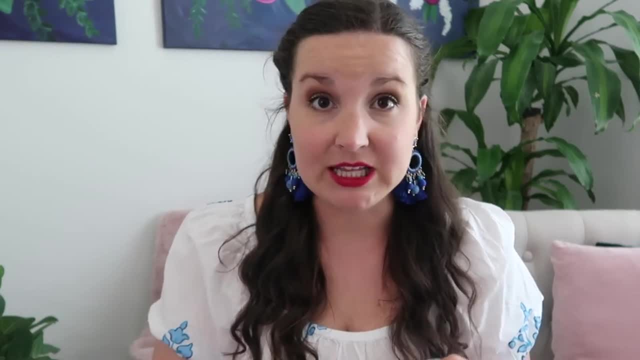 I make sure that you know I smile, I'm consistent in what I allow in my class, So if something got on Monday, it's going to get you in trouble today too. Like we're not, you know, wishy-washy with like. 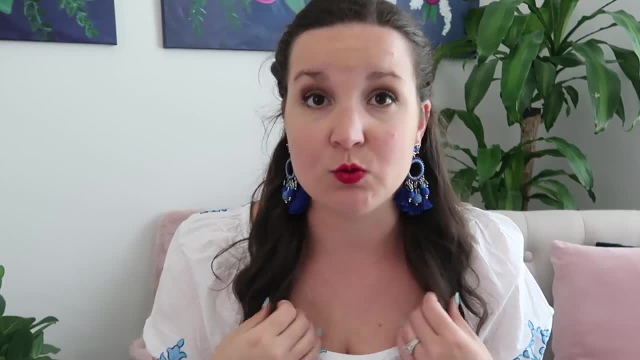 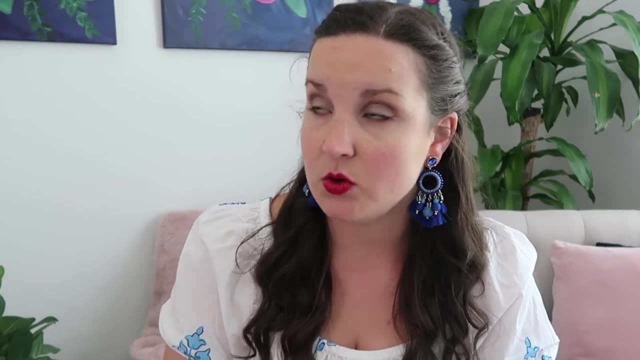 some days things are okay, some days things are not. I try to be very consistent with my demeanor so that students know what to expect. They're not like, hmm, is she going to be like an evil queen today? Or is she going to be like super nice and, you know, bubbly? I don't know, But I'm very. 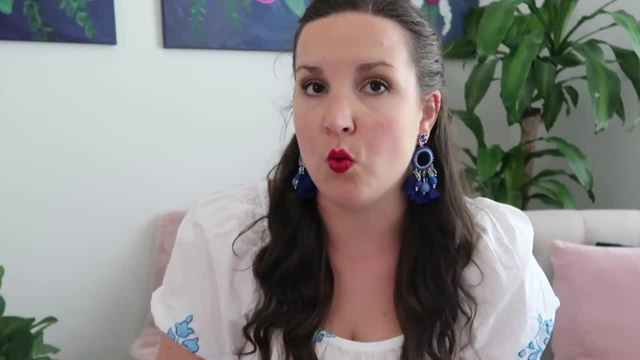 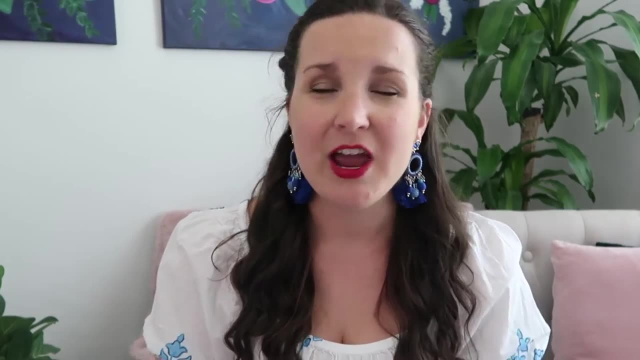 consistent with my demeanor, so that students know what to expect from me and they know what I act like. They know who I am. So then that helps them form the relationship with me, because they know what to expect when they come to me If they're not sure who you are, because some days you're like you know again. 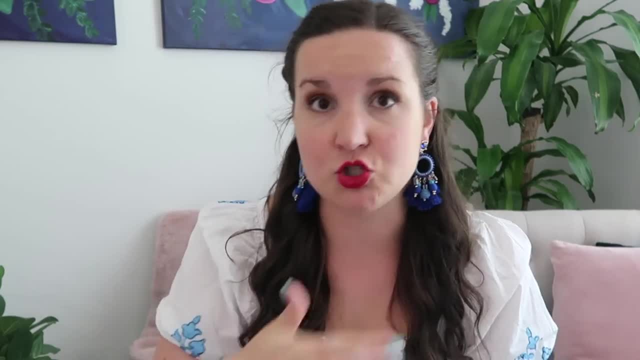 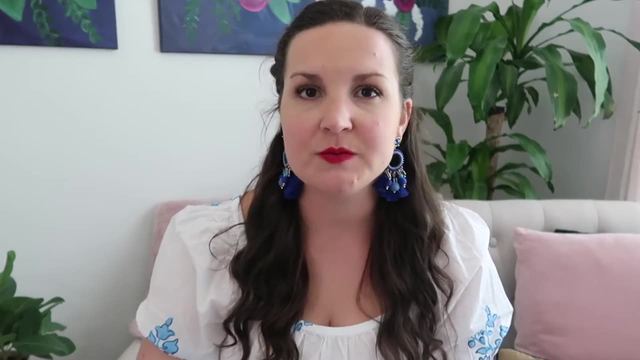 super frivolous, super fun, super bubbly, And other days you're like super mean and super strict. It's going to be confusing. So, just however you are, make sure that you are that way every day. Next up to help form relationships is make sure you look students in the eye. That probably sounds. 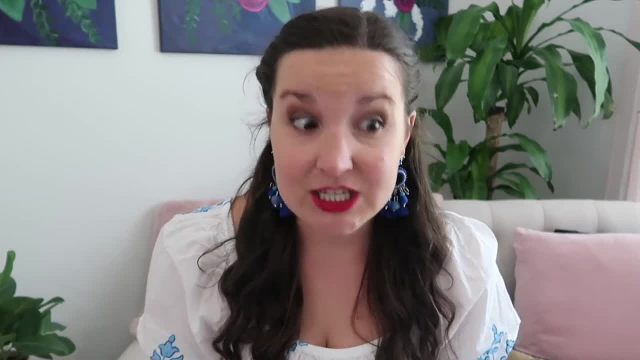 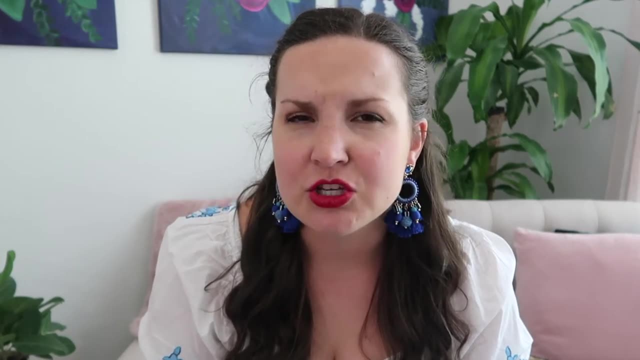 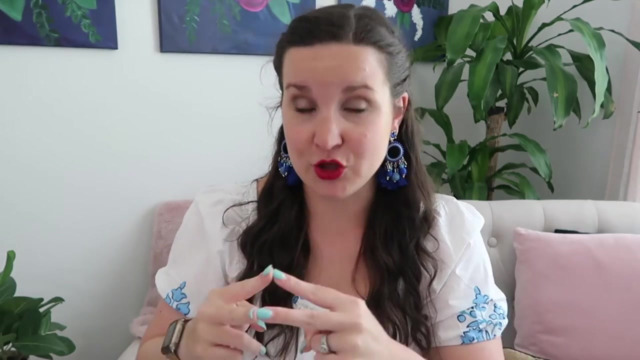 like the strangest suggestion, but it makes a huge, huge difference when you actually look students in the eye. I see teachers that, like never look their kids in the eye and it is the strangest thing. Forming eye contact helps you to literally connect with other people. So if you give them eye contact, 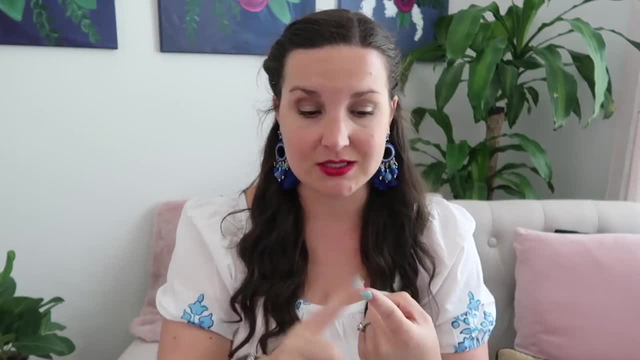 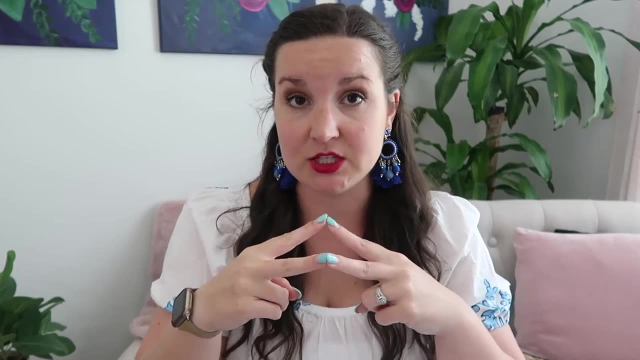 a little bit every day, then that's going to help them know that they are seen, that you see them, that you know that they are there, that you know who they are and all of those things that helps you literally connect with that student. I make a point to try to make eye contact with every student. 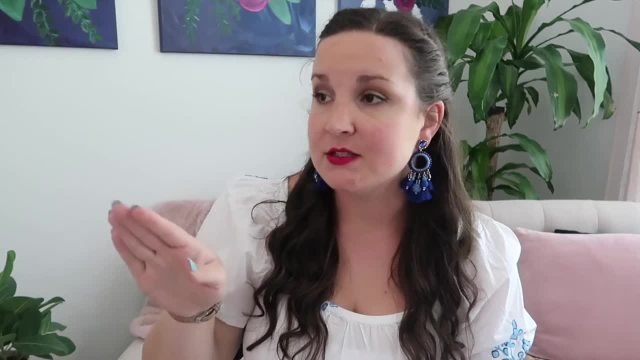 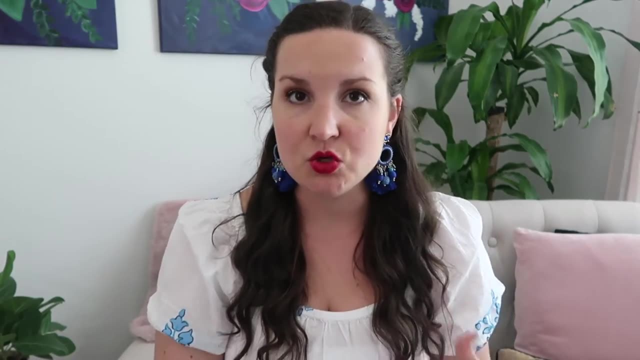 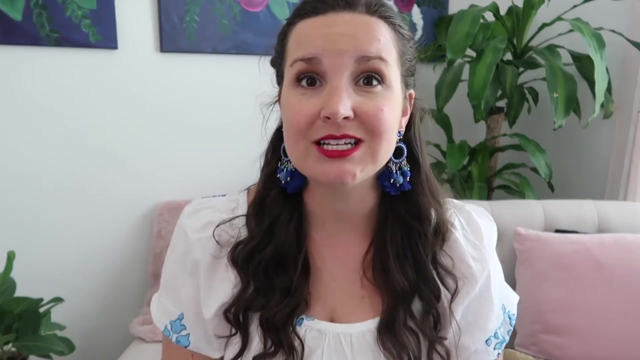 each day, not in like a creepy way, but like as we're singing a song. I'll look at each of the kids while we're singing And I make sure that I do that throughout class so that they know that they're seen, they know that they're heard, they know that I know that they're a person and all of. 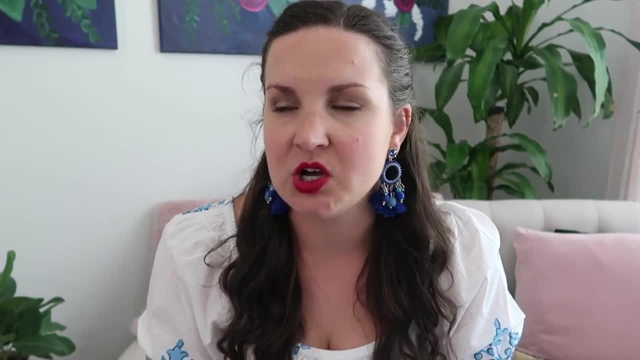 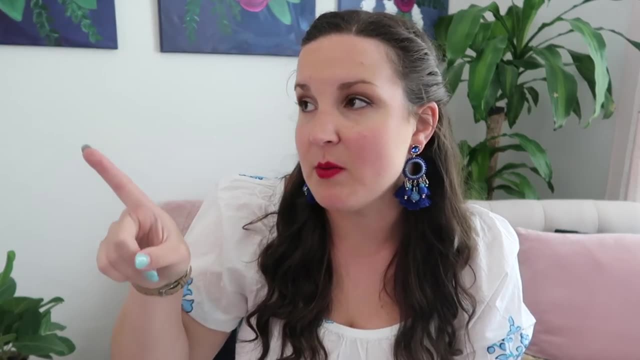 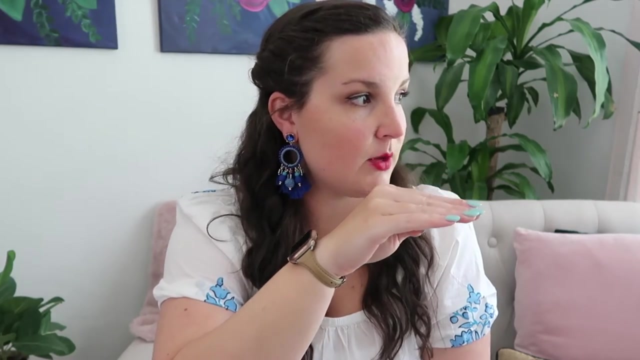 that kind of stuff. I once had a teacher who was in college but still he would, he would. I don't know if he like has stage fright or what, but he would take his eyes and his eyes would go up, over and down. He never looked at anybody in the eye. 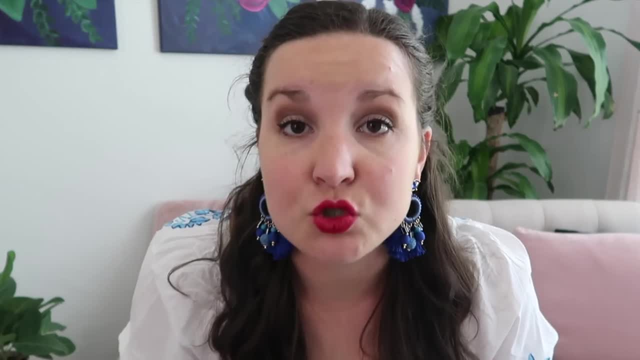 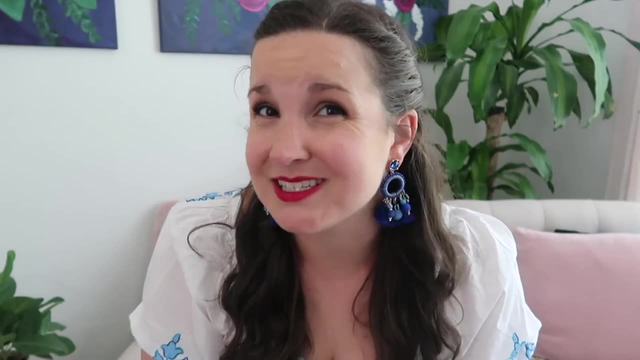 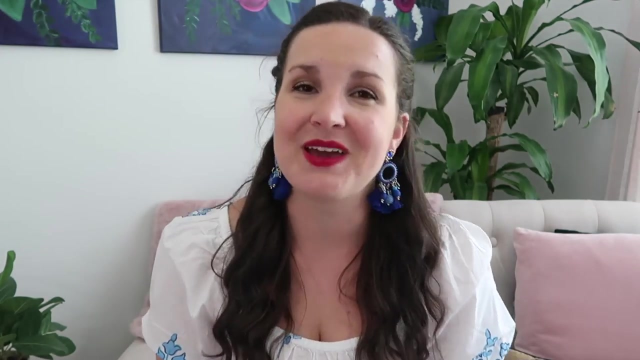 Just up and over and over And it was the strangest thing. And do you think that I formed any kind of relationship with him? No, I dropped his class because I was like this is super weird And also like, just in general, it was not my favorite thing in the world. So make sure you make eye contact. 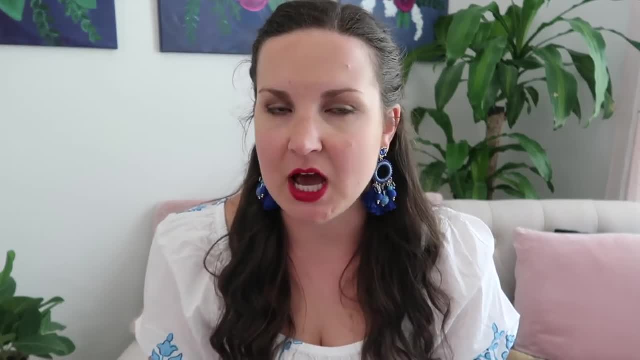 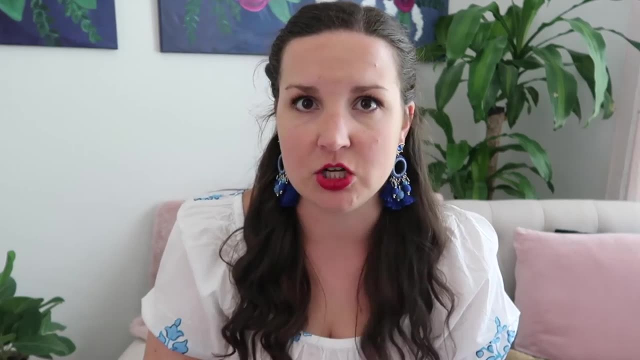 with the students and also encourage the students to make eye contact with you. I really, really started emphasizing that this year in particular, And I mean it's like your, I just finished year five, Um, but it made a world of difference, Like when you make a point to have the kids look at you and make. 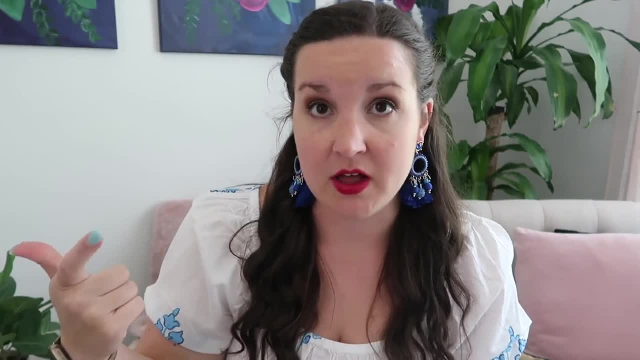 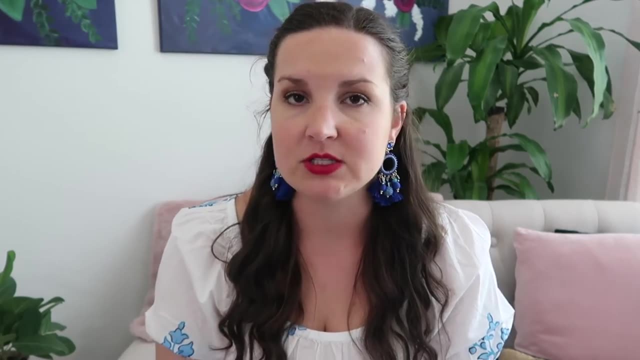 that eye contact, the focus, the class, the behaviors, the like. everything just gets so much better when you really make an emphasis, not in like a creepy way, but I always talk about having kids track me And I said, when you track me, you're watching my eye and you track where I'm. 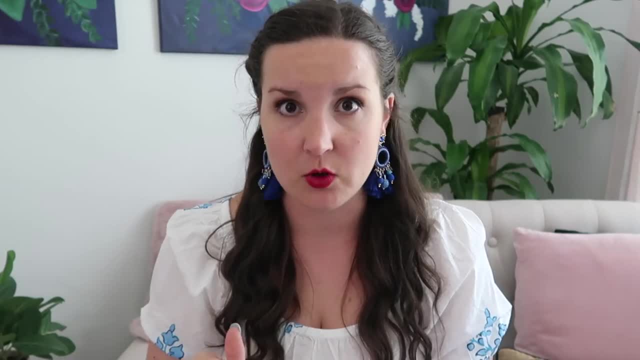 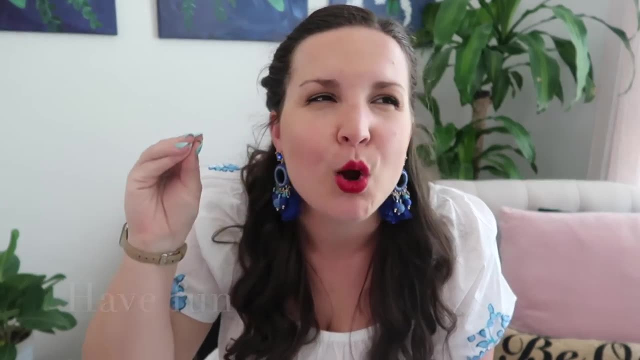 going and what I'm doing And that helps you focus And it helps me know that you're focused And that just really makes a difference. And the last thing that'll help you build relationships with the kids is to have fun. This is such an under rated tip. Nobody talks about this, or at least nobody that I've ever seen. 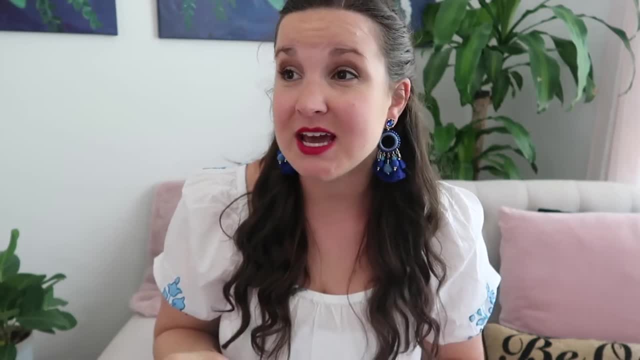 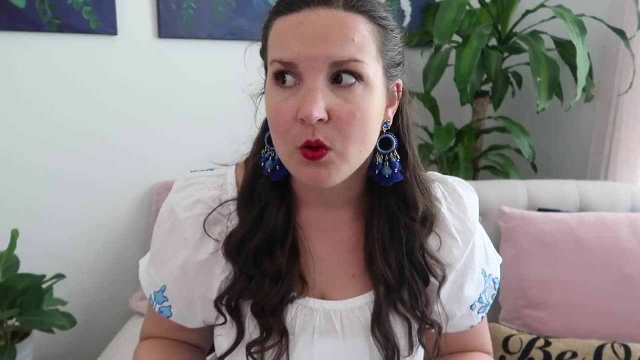 but this is so important: to have fun with your kids. Because if you think about like just normal relationships, like put it in just like a normal context, When you meet someone new, what do you do with them? You have fun. you go bowling, you go to the movies, you take walks. 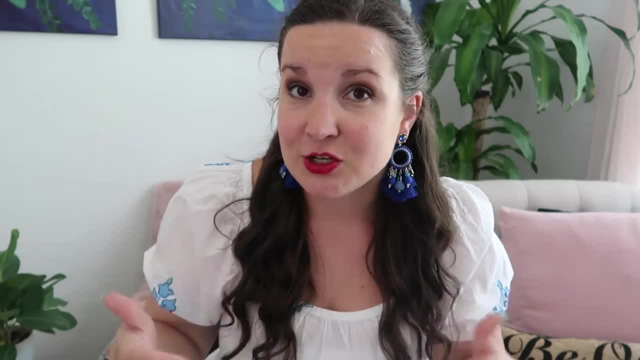 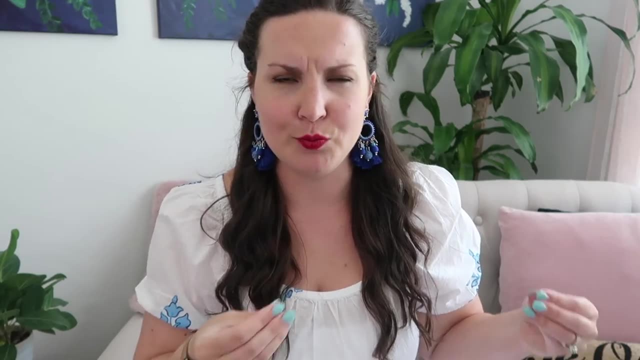 like you do things that are fun together. That's how you build your relationship with any person on the planet. When you were a kid, how did you build a relationship? How did you build a relationship with someone? You played with them. The same thing with your kids: play with them, play games. 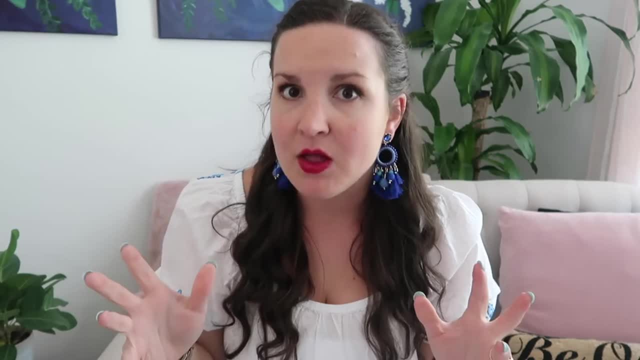 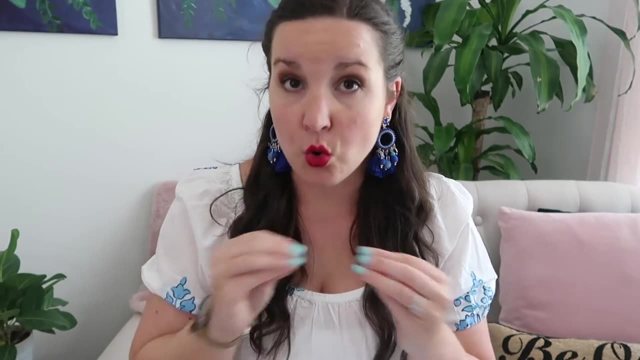 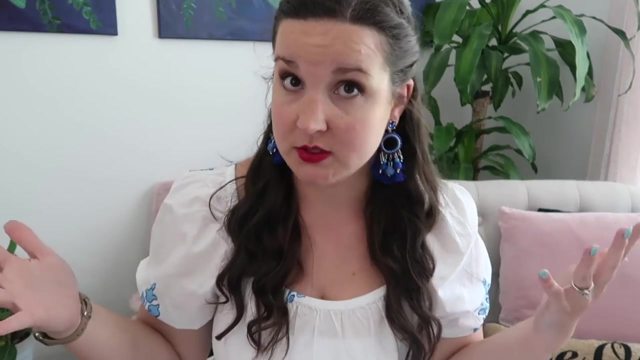 I would say, if you are new, spend the first solid like month playing games with your kids and really just having fun with them, Because that's going to create organic relationships with the students as well, as they're going to be like: Oh hey, music is fun, Miss Davis is fun, I like music. 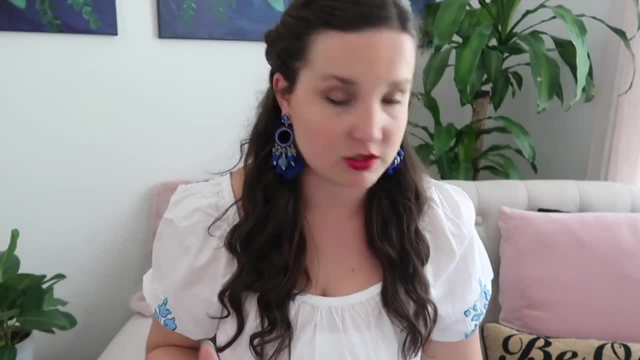 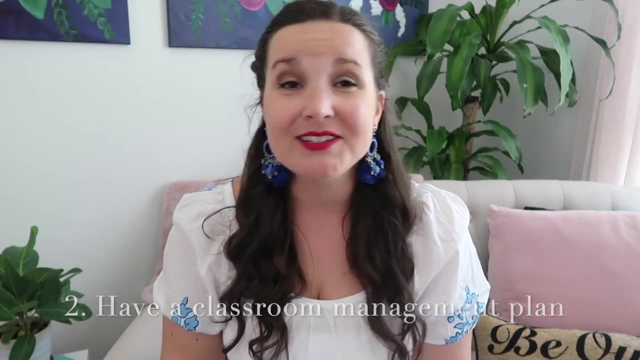 I want to come to music, And then it's gonna be a lot easier later on when I, you know, want them to do harder things later. So all right number two is to have a classroom management plan. This is something we didn't. 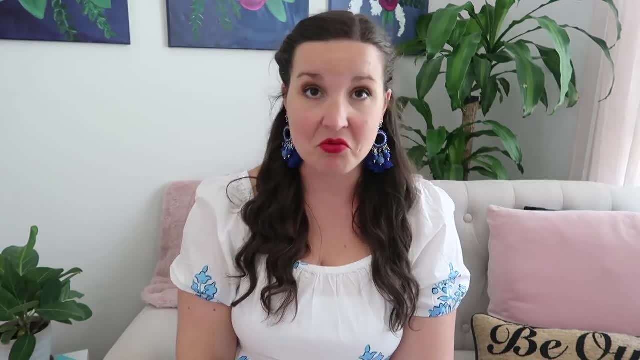 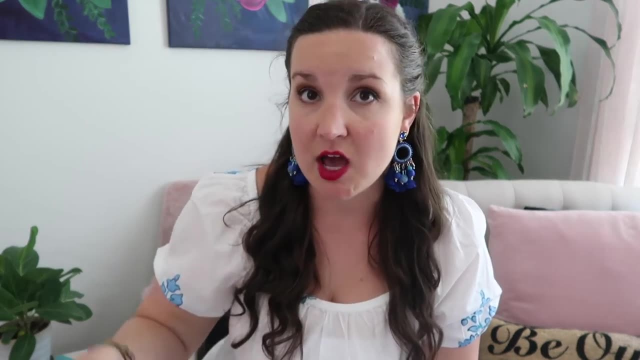 talk about at all in college And y'all. it is like the most important thing. the most important thing Because classroom management is literally how your classroom runs And if your classroom does not have rituals and routines and structures, it'll just fall apart. 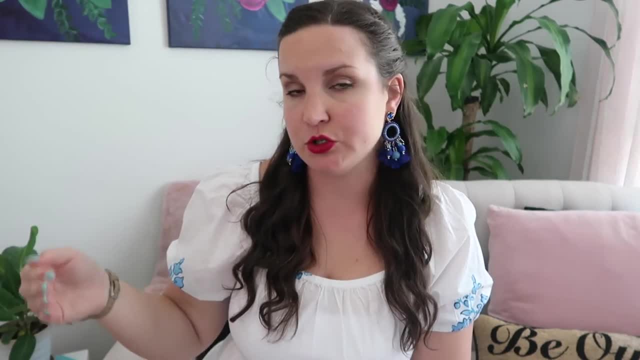 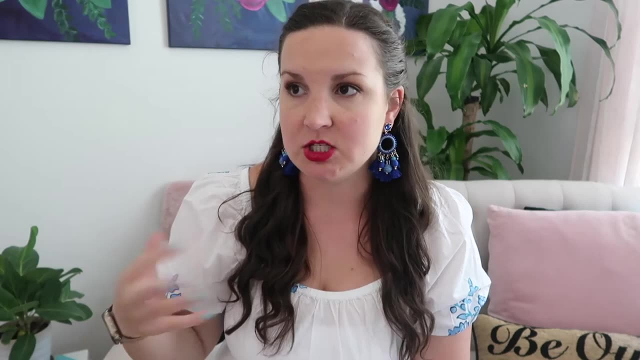 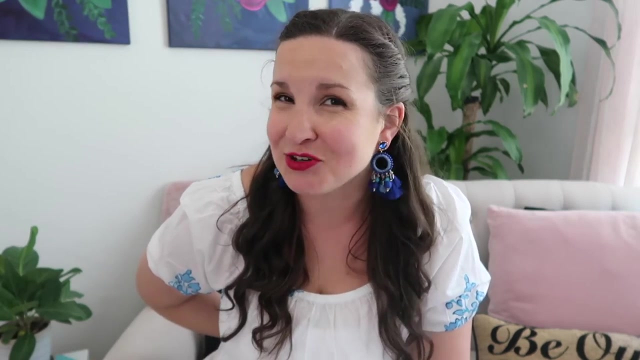 Yeah, I will also say: the more difficult your students are, the more you need rituals and routines and systems. Okay, I actually was teaching summer camp this morning, filming this over the summer, And I have a particular class that is extra fun, And so with them, I made sure that we had extra layers of 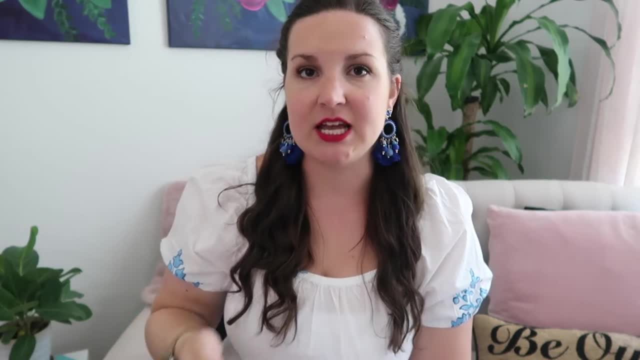 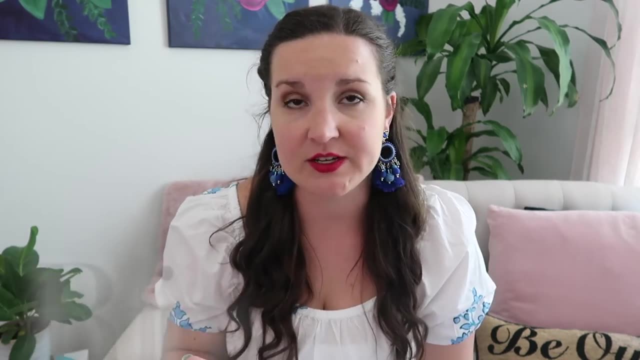 structure in class and just extra layers of things to make life easier. Now, with your classroom management, there's a lot of different things that go into it. you're going to need one: routines. routines are going to be things like: how do the kids do their homework? How do the kids do their? 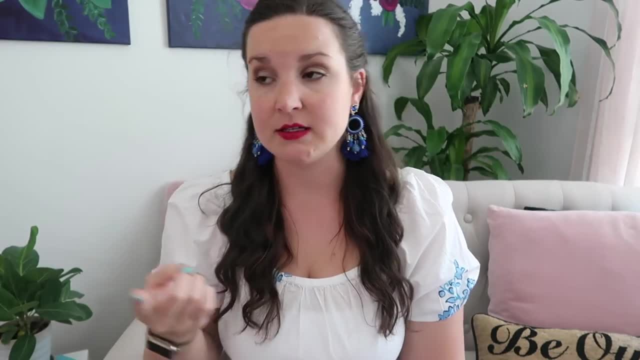 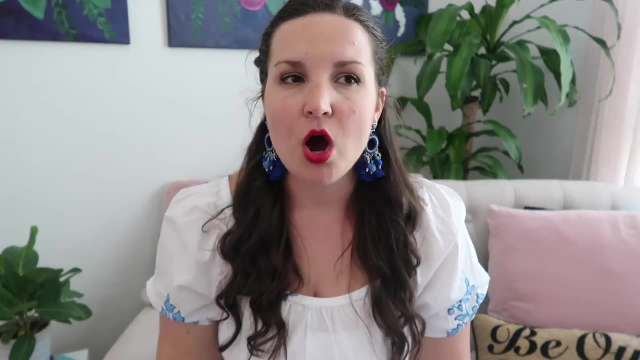 homework. How do the kids come into the room? How do kids leave the room? Can they go to the bathroom during class? How did they get to go to the bathroom during class? What do they do if they need supplies? How do you pass things out? All of these different things are rituals and routines. 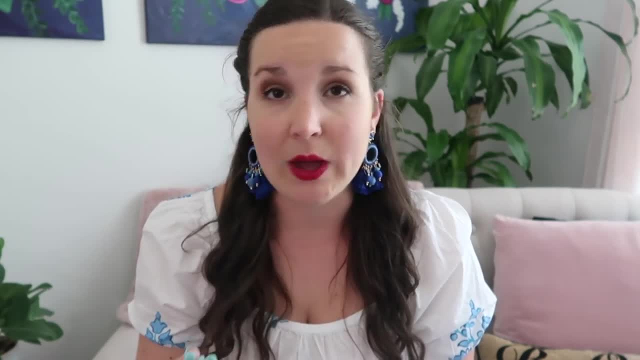 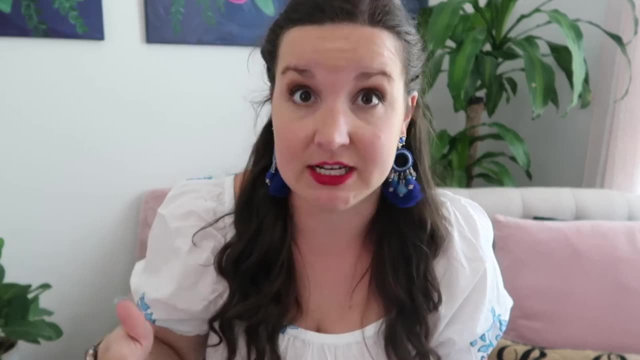 that you need to have in your classroom. Now, the good thing is, there's not like a magical way to do them, So it's not like you're right or you're wrong, It's just that you need to have an idea. 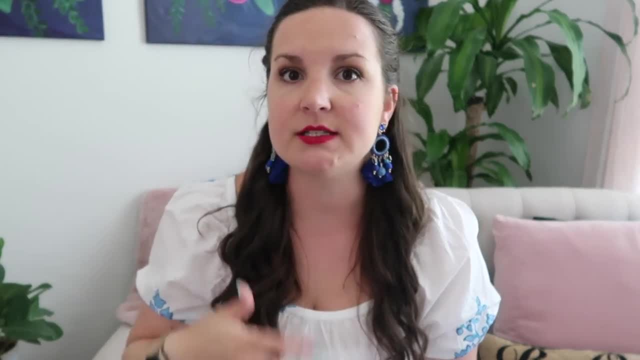 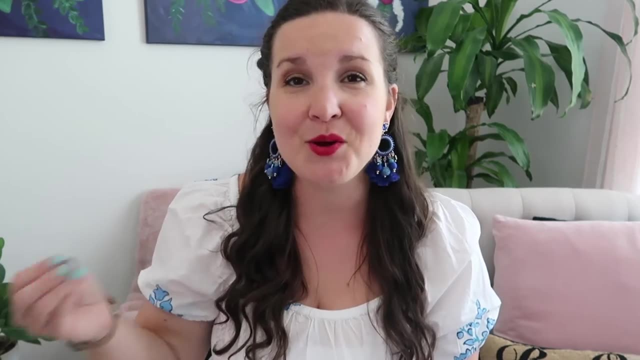 you need to have a plan Again. how are the kids going to come in? Where are they going to sit, Like, what are they going to do? Do they need to raise their hands before you to ask a question? Like those kinds of things. just decide ahead of time so that you know and they know what to do. 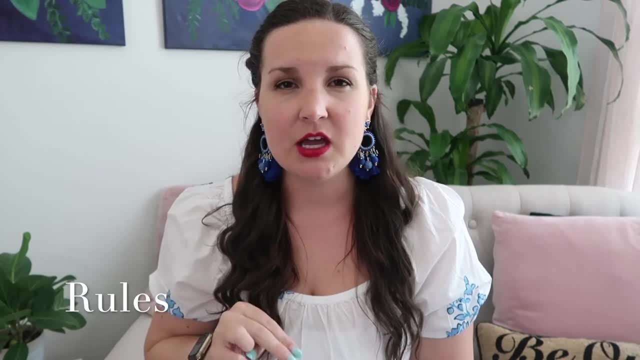 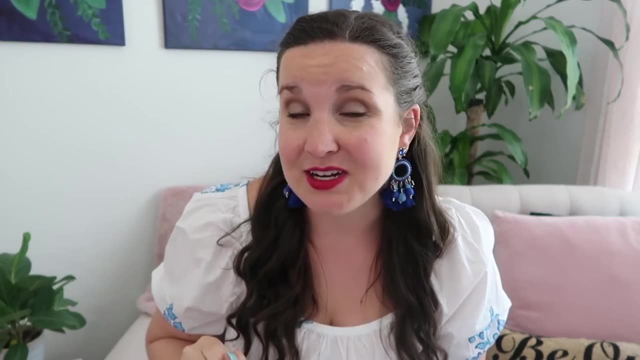 Number two is you're going to have to have a couple of rules. I'll link a video about how I teach the rules down below, but I just have four and they're follow directions: be respectful, be responsible, be a participant. I'm going to be honest. we could probably boil it down to just 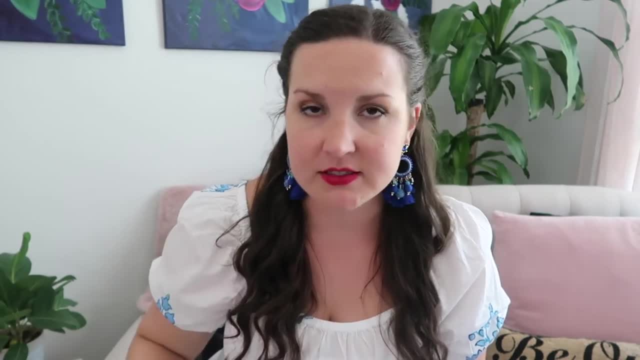 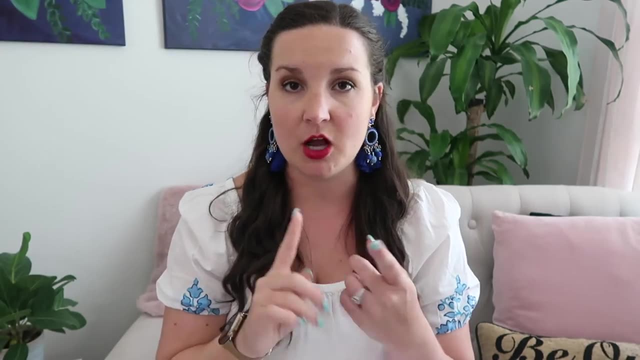 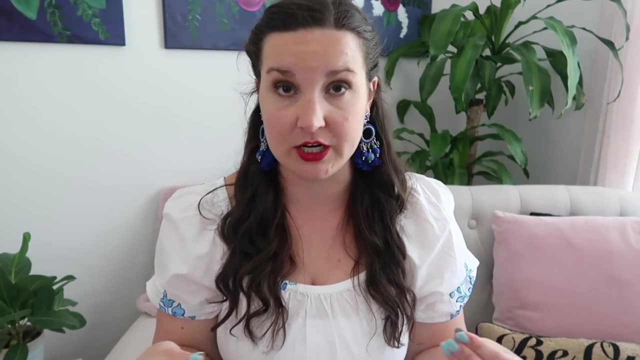 be respectful and be responsible and everything else would fall into place. But I do like having the other ones more specifically, but not just having the rules, but also making sure that you like to talk about what they mean And in context of different things. So when we do an activity, we talk about how we're going to do. 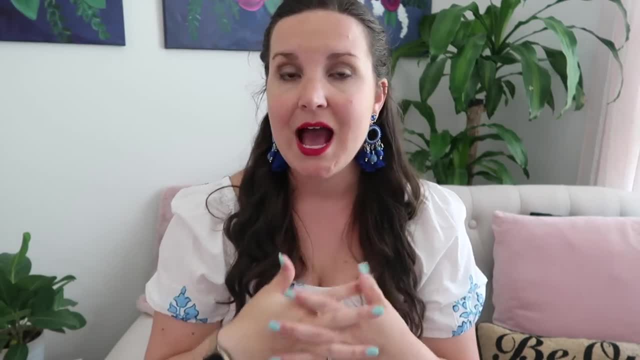 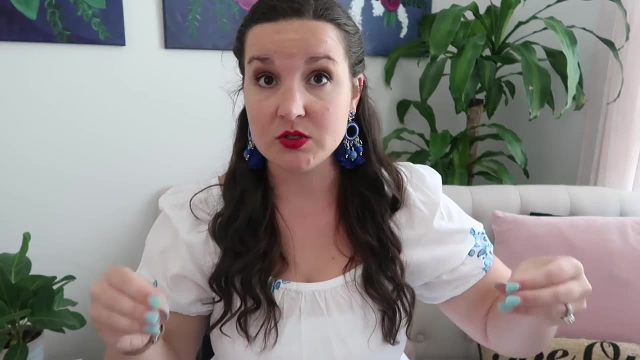 that. So if we're playing a game that requires moving around the room, okay, how are we responsible as we move around the room? Do responsible people run? Do responsible people break things? Do responsible people you know touch things they shouldn't Do. people who are do respectful people? 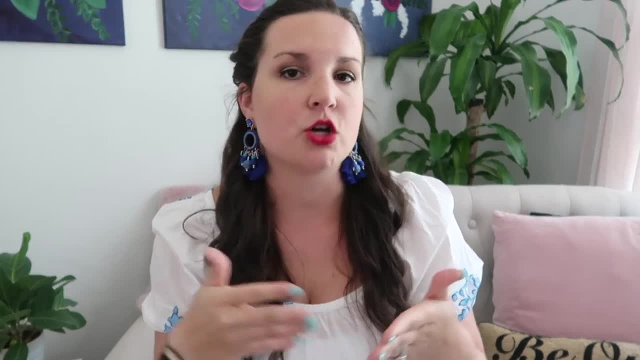 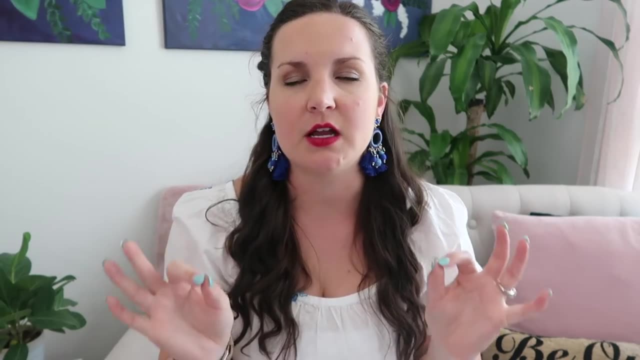 push people Like we go over those things, that I use the actual words that are in the rules to make sure it all comes together And we talk about that like literally with every activity, And I know it seems excessive but it's not. 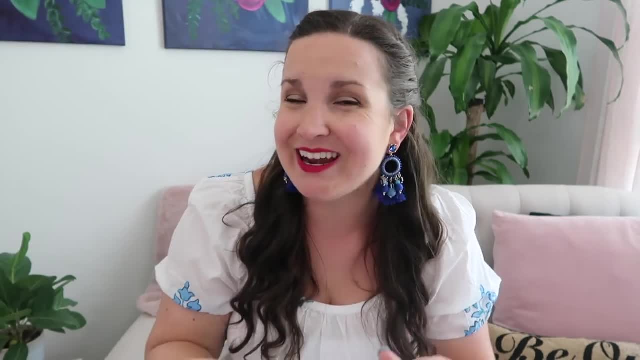 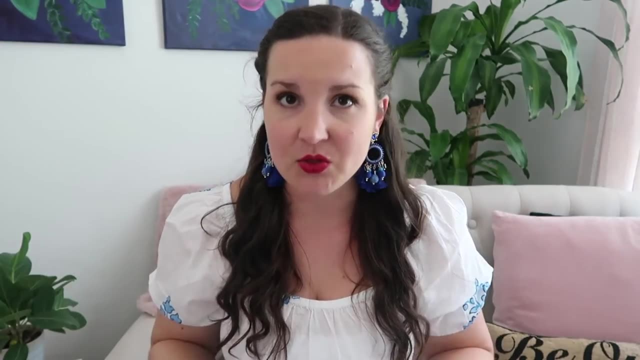 especially at the beginning. If you can like, drill it into them at the beginning, it'll get easier. Like we're at the point now that I've had my kids the whole time they've been at our school And so, like my fifth graders, they know the rules, they know what to do. I don't 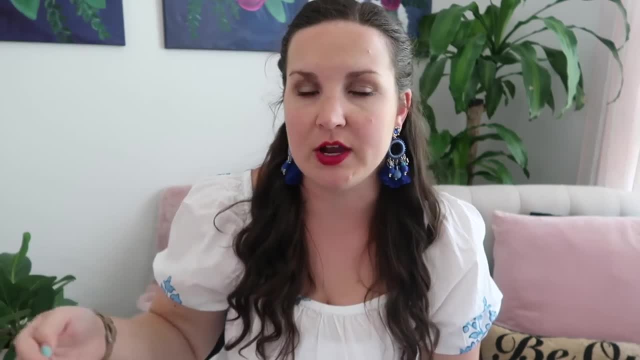 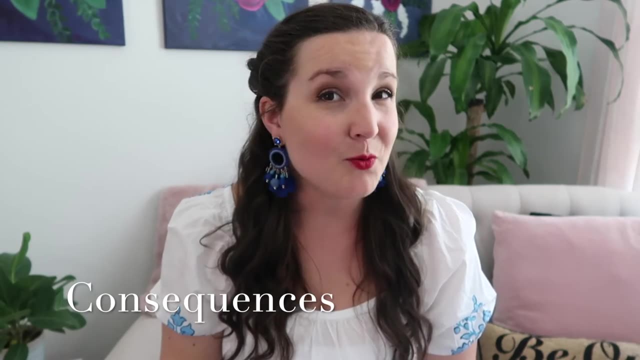 have to spend as much time on them because they have it so ingrained in them- but especially at the beginning- really, really, really make it a big deal. Number three is consequences. If the kids are not following directions, then what's going to happen Again? 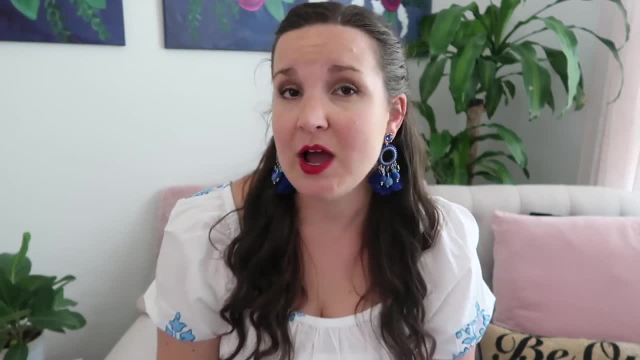 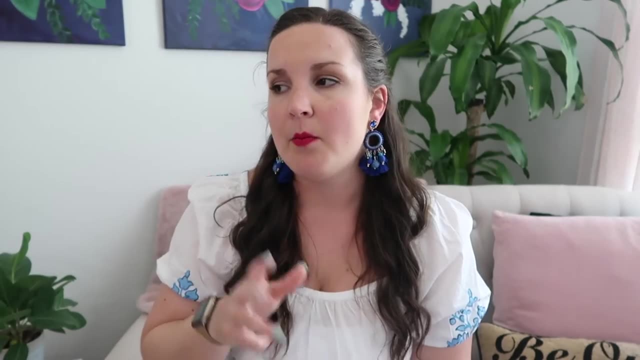 not like right and wrong answers, but there needs to be something. So I will link a video down below about like classroom management and how I deal with all of that, in case you need like more ideas of that. But yeah, I will link a blog post down below. There's a video that either already came. 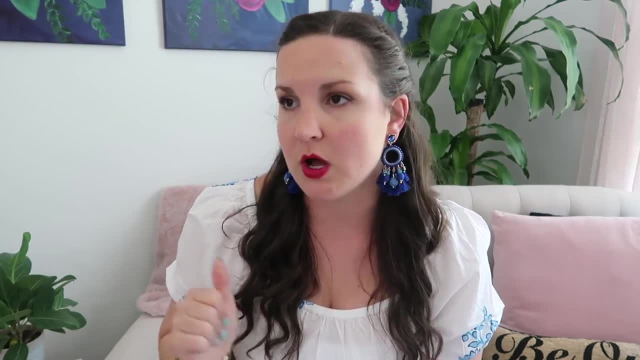 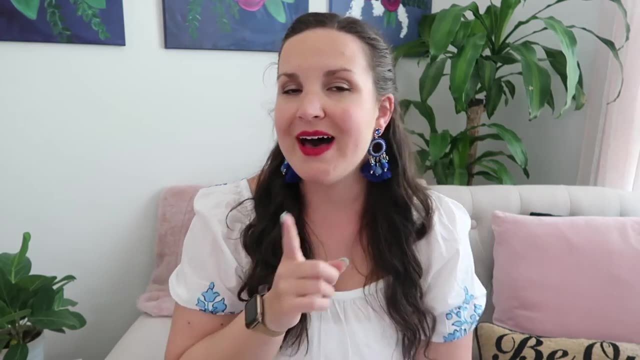 out or is about to come out. that goes along with the blog post. So if you prefer to watch that, either it is available or it is coming. I have, I don't know. I have it written down somewhere but it's not in front of me And in this video. 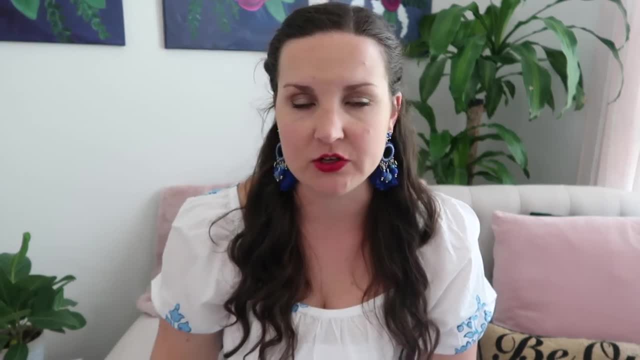 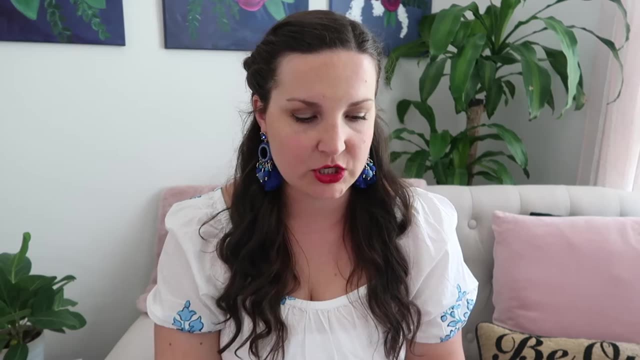 it's about the consequences for in my class, What happens if you are not following directions. They're very easy, They're very simple and they work for me and I've been using them for years, so I would recommend them, But just making sure that you have some kind of plan. Number four: 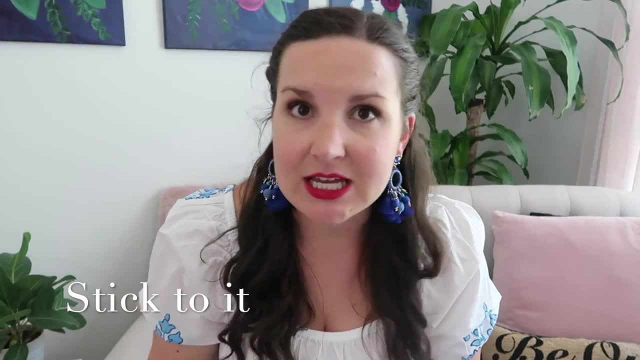 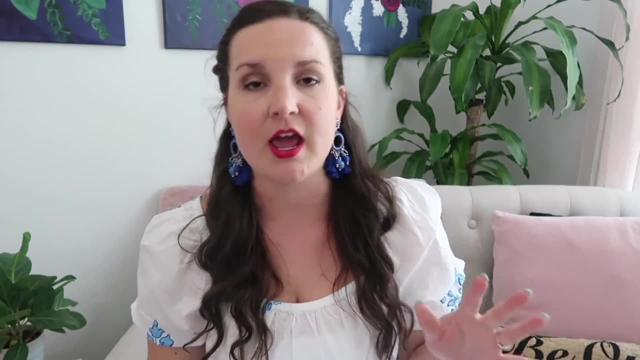 when it comes to classroom management is: stick to it. Do not be like super classroom management person one day and then like super willy nilly the other day. You have to be very consistent in what you expect so that the students know what to expect, so that they will do it If. 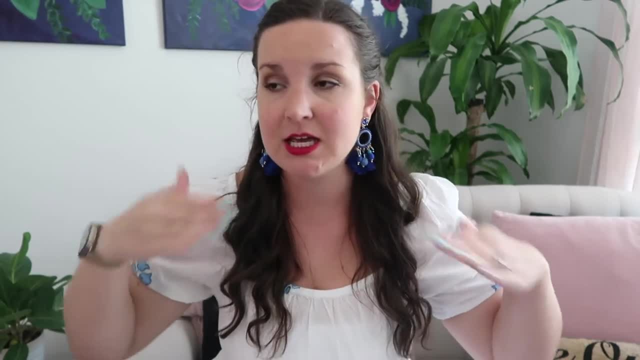 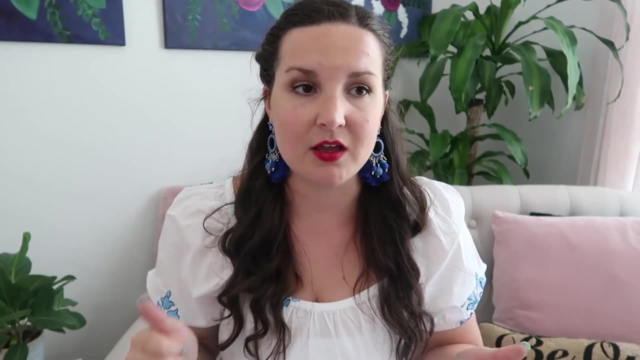 you sometimes give consequences and sometimes don't, the kids will not respect you One. they will also not know what to do And they also just like- I mean literally, like you can see it, It's really depressing. You'll see some teachers that completely lose the respect of their kids. 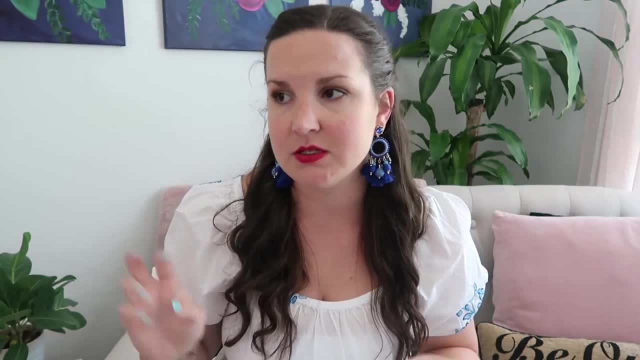 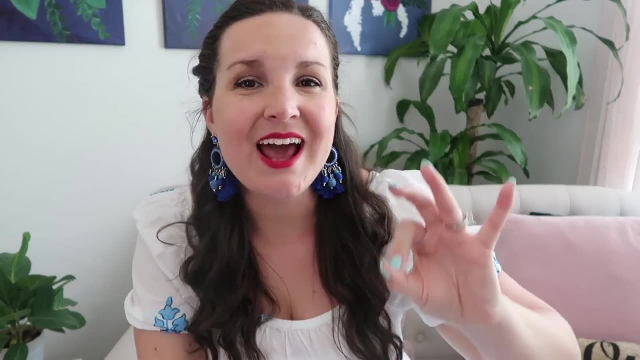 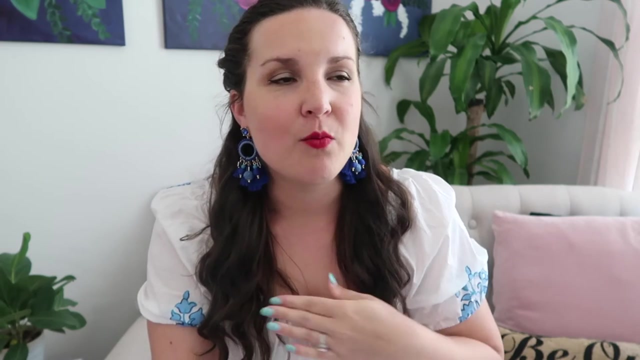 And it's usually because they're willy nilly with their consequences or they don't treat them like humans. So there's, there's two things, And number five is: explain absolutely everything in excruciating detail. The longer I've been teaching, the more I realize that it's not necessarily the kids want to be bad. 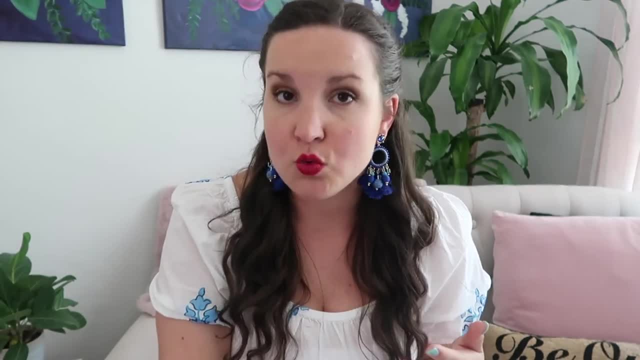 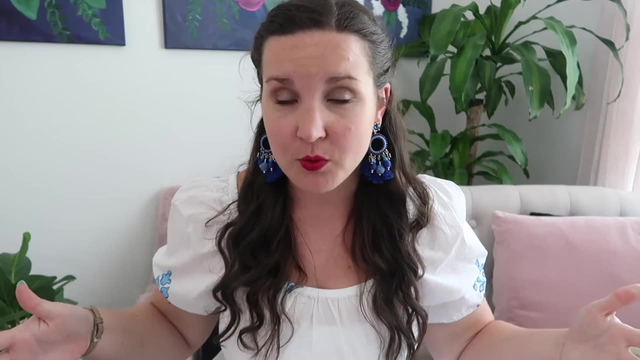 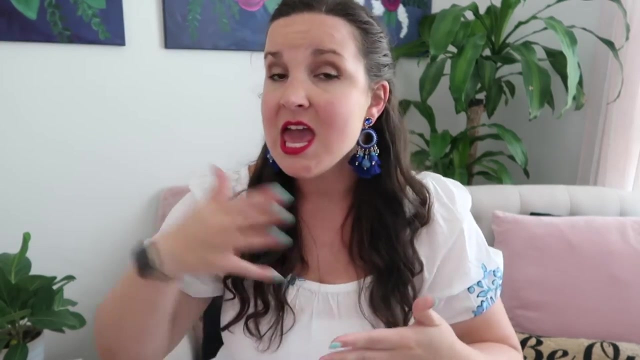 A lot of times it's just that they don't know what to do or they don't know that they shouldn't do something. So make sure that they know what they can and can't do. If we're moving around the room, then I need to be explicit about where we're moving, how we're moving if we're touching. 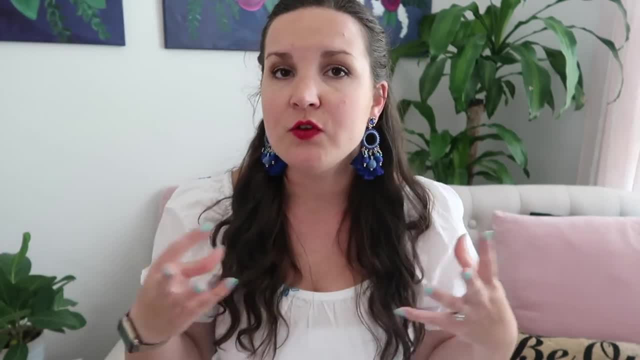 things, if we're not touching things, if we're running, if we're not running all of these things, And I think that's really important. And I think that's really important, And those things need to be discussed And they need to know in excruciating detail exactly what to do. 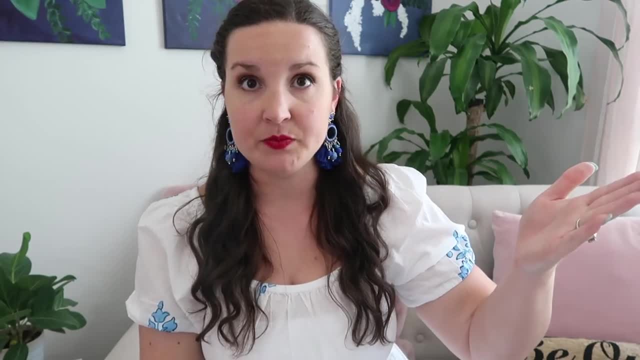 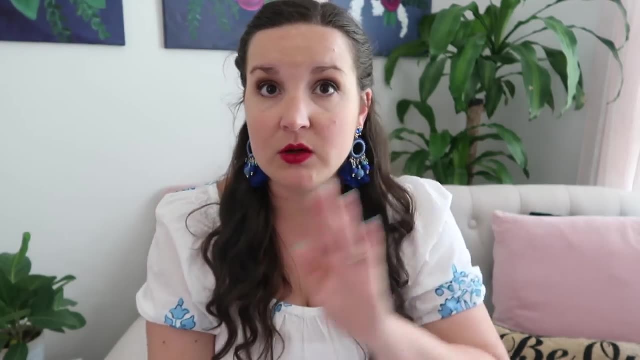 If we're lining up and I just say: get in a line, that might be all sorts of wonky, with people talking and hands everywhere, Versus if I say: Okay, the green row, stand up, walk this way, stay. 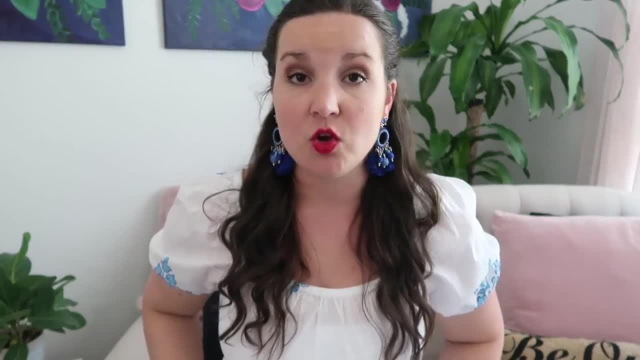 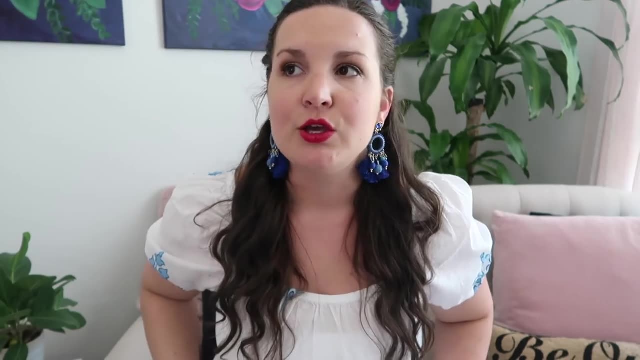 in your line, get in line. your hand should be in your pockets, your voice should be at level zero, I shouldn't hear any noise. Those are very different things And the more detail you can give the better, especially with the younger kids And especially at the beginning. 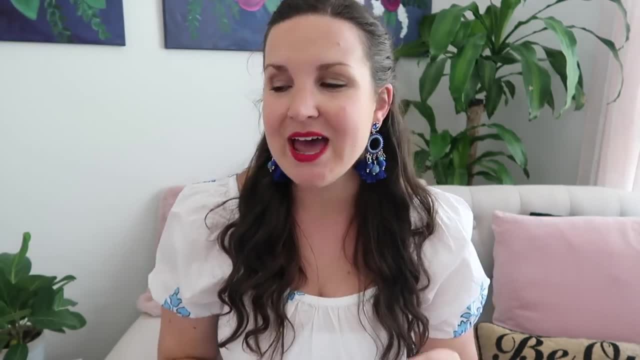 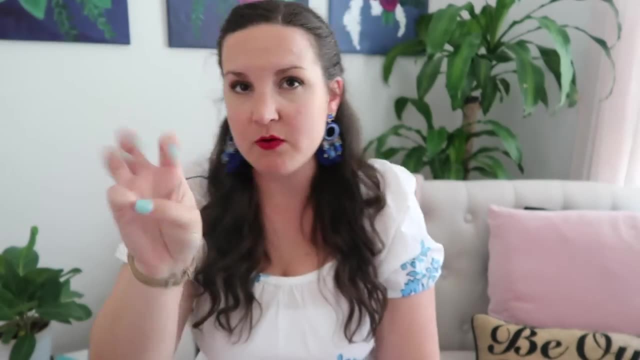 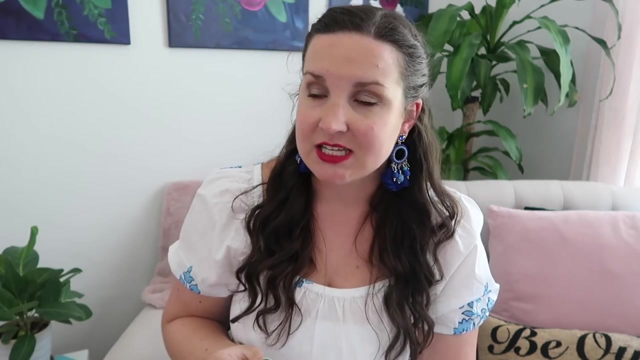 again. if you drill it into them at the beginning, it'll be easier down the road, But it seems excessive And it is. do it anyway. it'll make your life so much better. My third tip for new music teachers is you have really quick paced lessons. The easiest way for kids to get off task is when 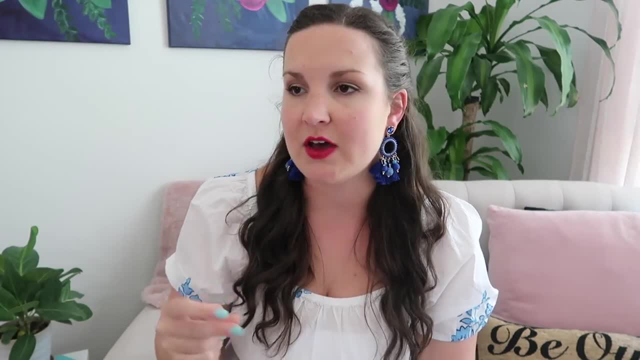 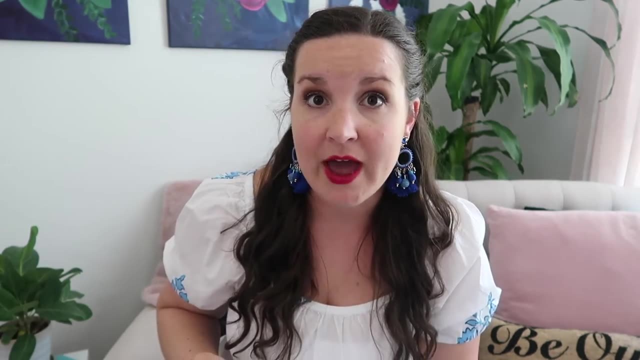 there is a long transition between different activities. So the faster your places, so the faster your lessons get done, the faster your music teachers get done. So the faster your lessons get done, the better. Don't give them time to get bored, Don't give them time to act up. We have 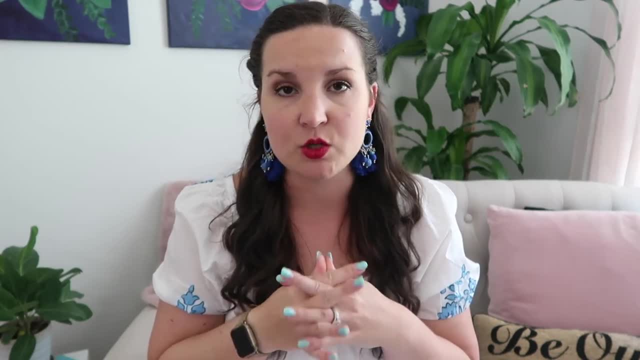 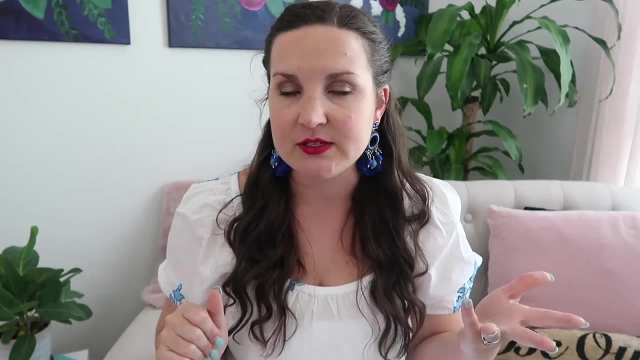 very short things. When I was in college, actually, we talked about attention spans of students And the chart that I was shown said that basically, kids have about the same attention span as their age. So if they are five, they have about five minutes of an attention span and nothing more. 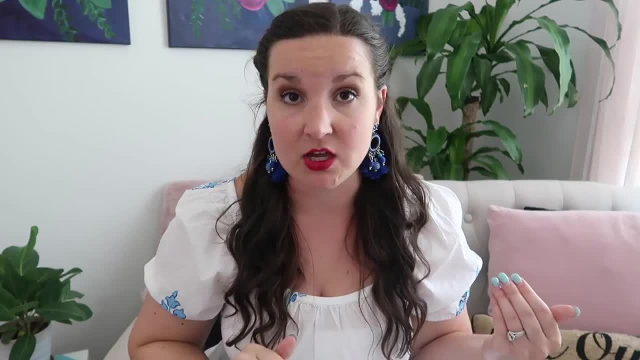 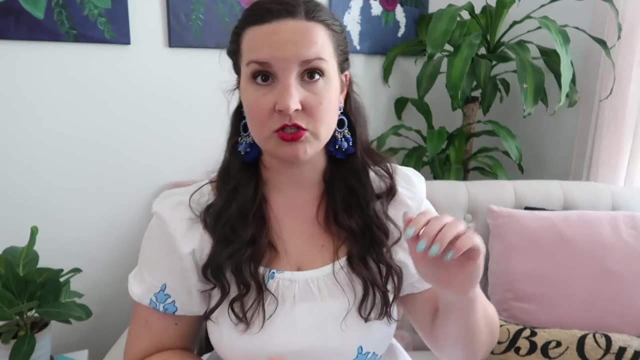 So if you're doing an activity, it needs to change every single five minutes in that kindergarten class- And I know that sounds like a lot- do it anyway. So with that, we're doing a song, we're doing a game, we're doing another song, we're listening to. 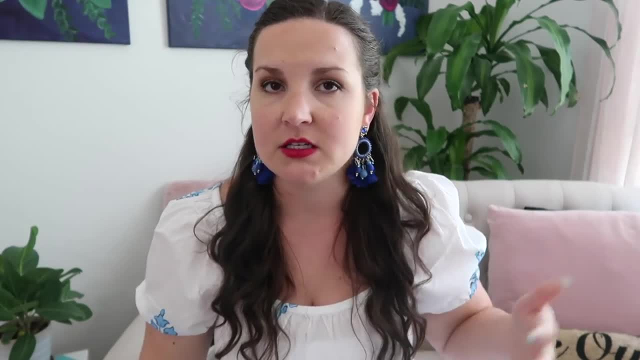 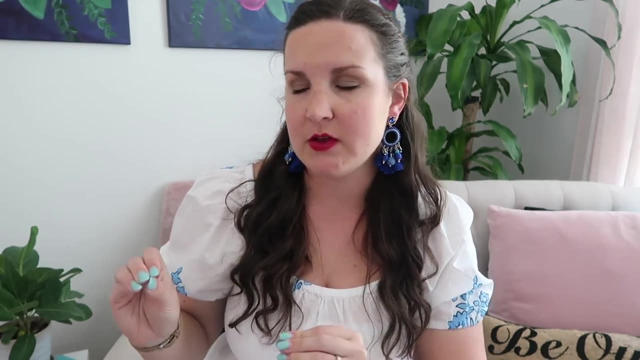 a song, we're moving all of the different things, But make sure that the lesson is going quickly so that they don't have time to get bored and they don't have time to act up With the older kids. I feel like you can fudge it a little bit if it's fun. So if my older kids are 10,. 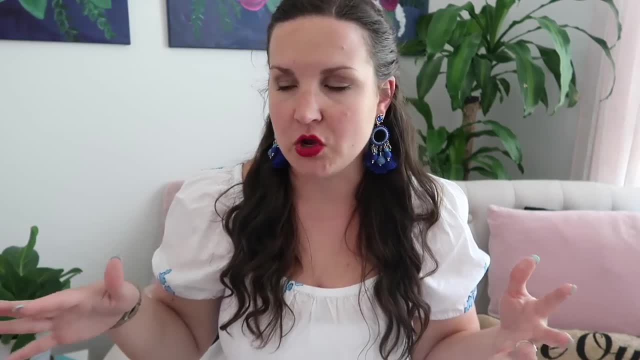 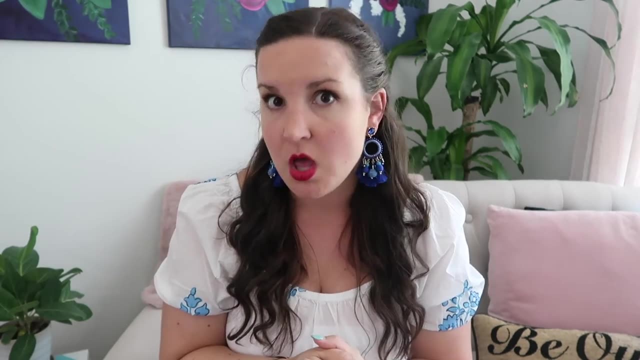 usually I can get 15 minutes out of them, but not usually any longer than that. So, making sure that your lessons go really, really quickly and that you minimize the transitions as much as possible, Don't take a huge long time to go from one activity to another, or just go. 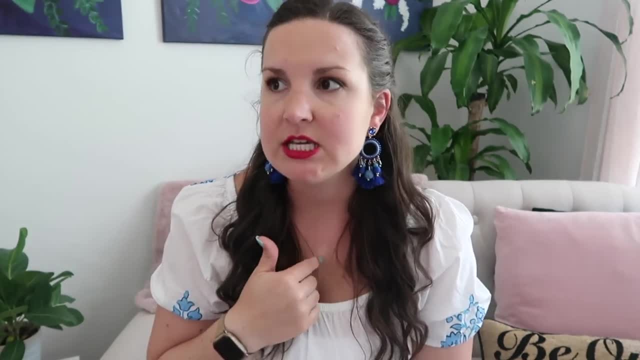 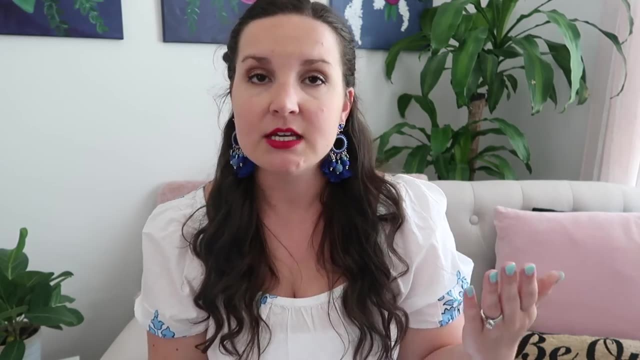 straight on in. One thing that really helps me with that personally is that I have Google Slides for all of my lessons, And so I have, you know, like, okay, third grade on Wednesday is doing this, this, this, this and this, And they're Google Slides. I have a little clicker I got. 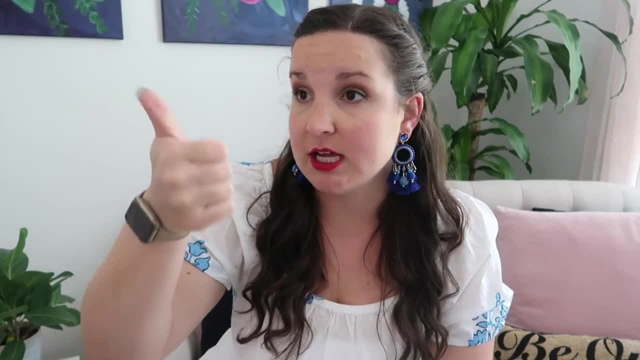 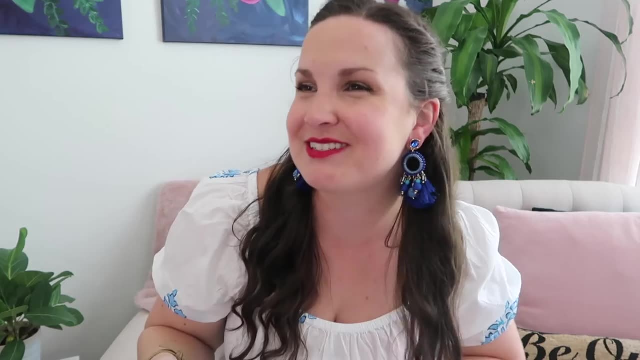 from Amazon for like six bucks And I just click through. I'll link it down below. It's really handy and really cheap And I've dropped it multiple times and it has not broken. So that's also helpful in elementary music. So I just click through them And so. 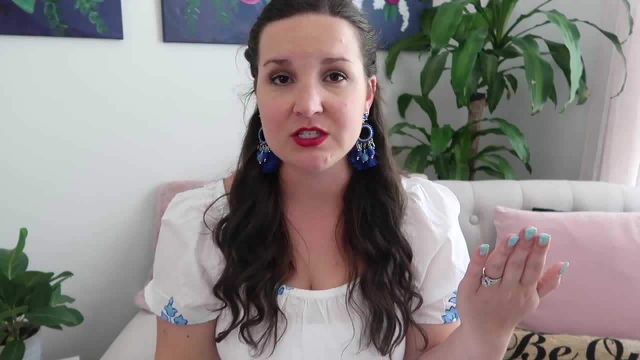 it'll have you know like, okay, now we're doing Twinkle Twinkle, Little Star, Here's all the words, Twinkle, Twinkle, Little Star, And then I have, you know three questions I wanted to ask. 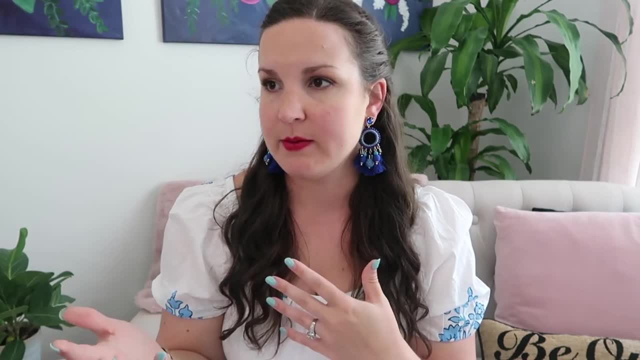 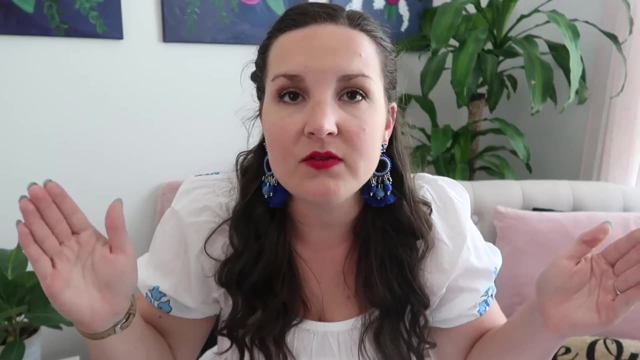 Here are the three questions. And then you know, like maybe we're listening to a song And so I have a Google Slide with the song we're going to listen to, or maybe I have the YouTube video invented because that will change your life, And I mean seriously. sometimes it'll be just like 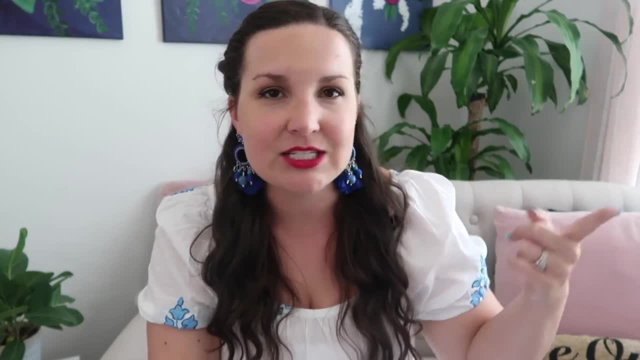 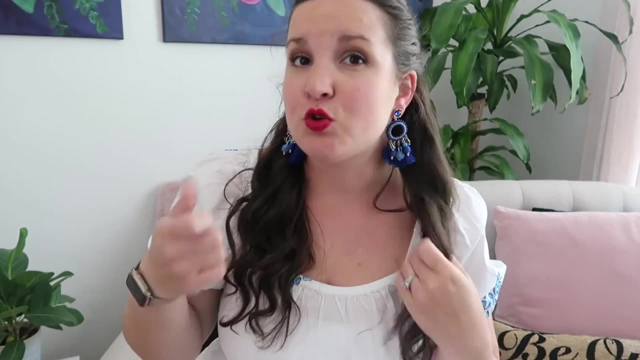 a triangle, but it will remind me that I need to do something that has to do with triangle, Like, maybe we're going to talk about the triangles, I don't know, But having a slide really really helps me to remember where I'm going, so that I eliminate. 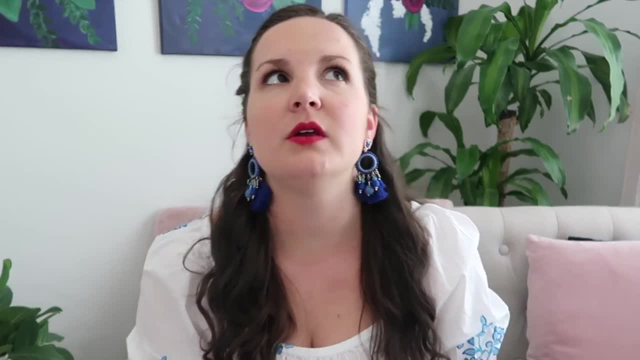 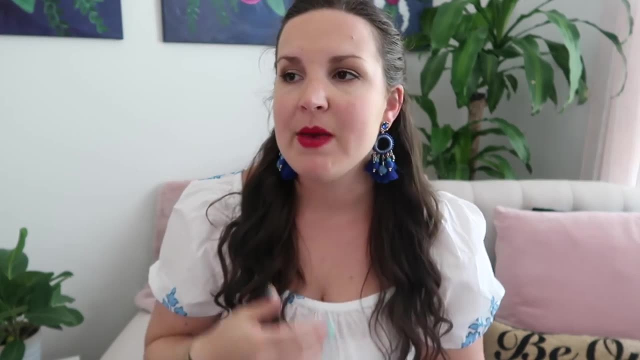 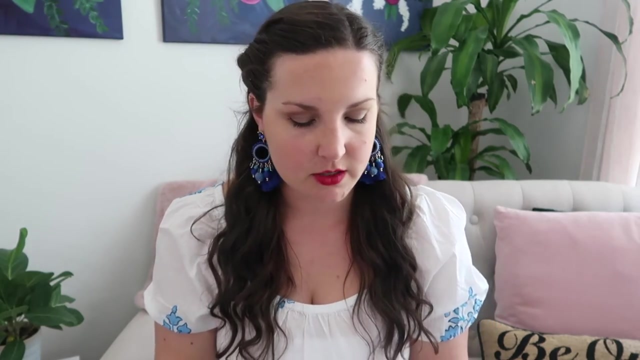 all of that Like what are we going to do next? I don't remember. I just go click: Oh, we're doing that song next. Excellent, Let's go. And it just really helps to me, like personally, to change pace Really. let's be honest, The slides are for me, They're not for the kids. 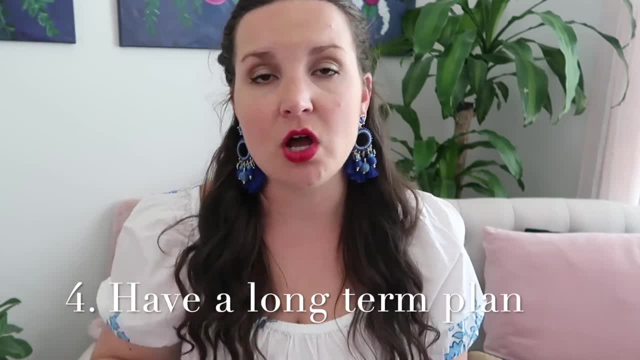 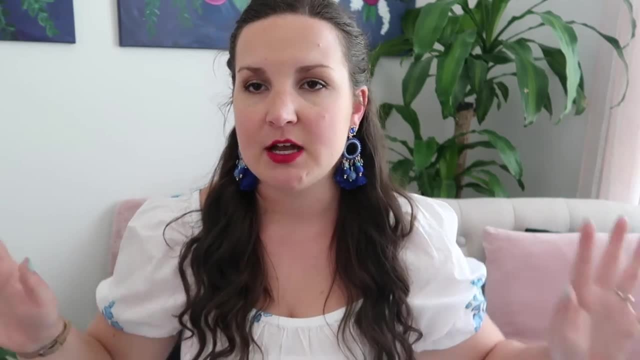 but still. Number four is: have a longer term plan When it comes to teaching. you do not want to be a week to week teacher. What I mean by that is being like sitting down and be like: all right, I need to have a lesson plan for next week. 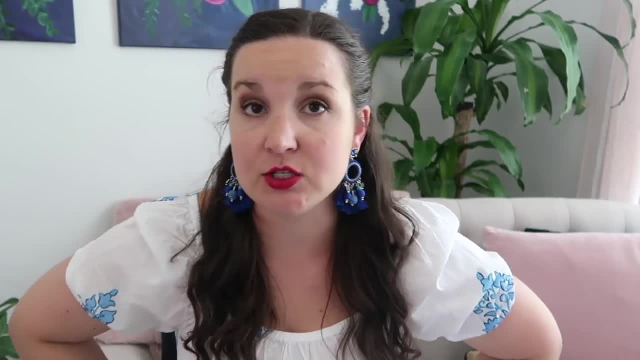 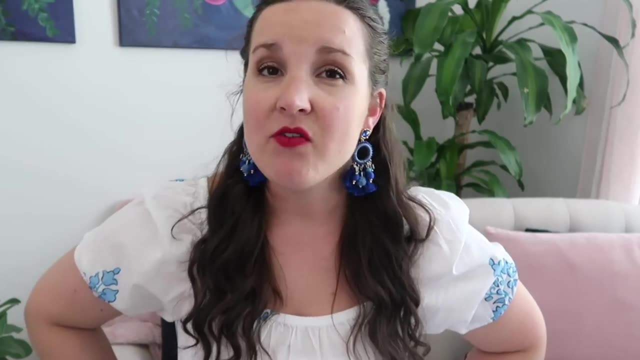 Okay, We're going to do this random thing, And then the next week we do this random thing. The next week we do this random thing. No, no, no. Have a longer term plan of what you're going to teach. I have a whole video about how to create this. It's called a scope and sequence. 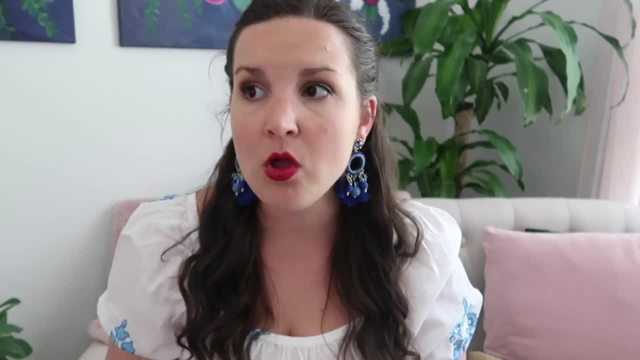 I will link it down below. Go check it out because it's really really helpful. We also talk about that in the free mini course, which I will link down below. So if you're interested in that, we'll also link down below, if you want, you know, a little bit more help with that. 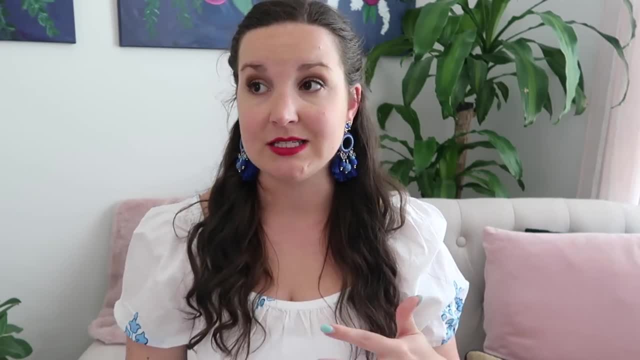 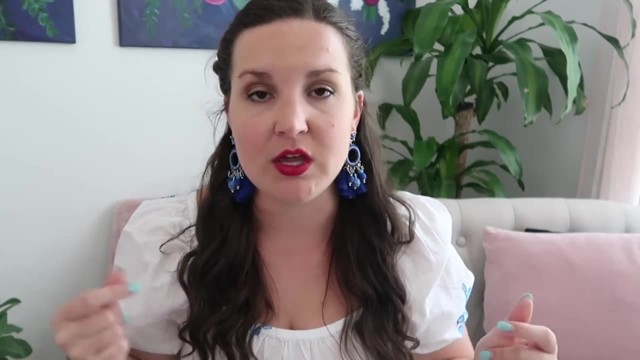 But having a plan long-term will just make your lessons go more seamlessly because they will fit together better, And it will also help you to get out of the week to regret, because you'll know what to do If you're like. okay, we're teaching quarter and eighth notes for the next three. 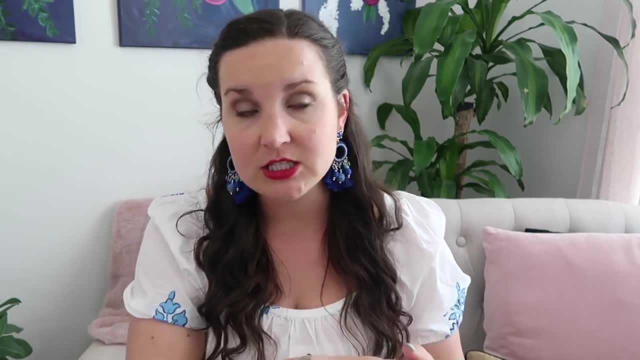 months. Then I have three months worth of things and I can make sure I spread out different activities throughout there. You don't have to have three months planned out, Just have like an idea of what you're doing at what time. So if you're like, okay, I'm going to do this. 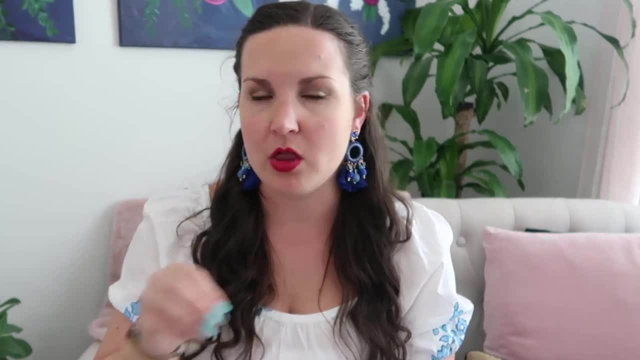 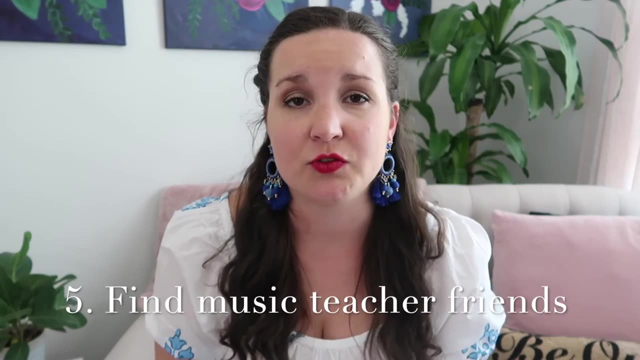 so that you know kind of what to do again, I'll link a video down below with all of that and like a sample sequence and everything to help you with that situation. Number five is find some elementary music teacher friends. This can be difficult but it's also really, really, really really helpful. 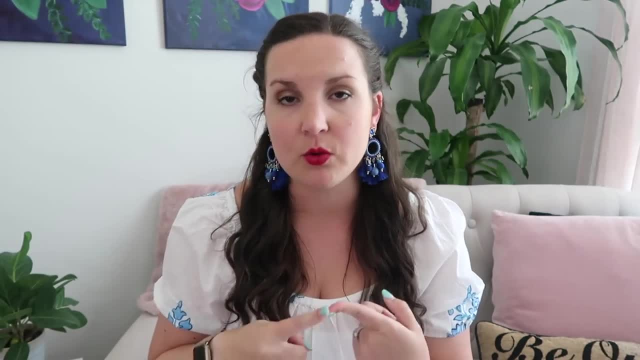 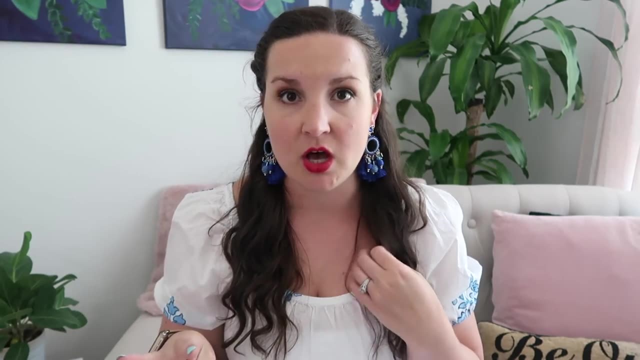 how to find elementary music teacher friends. If you graduated with different people who are doing elementary music, connect with them. I, it's been again five years and there's still four of us that taught that teach elementary music, that all graduated within like five years. So if you're like, okay, I'm going to do this, I'm going to do this, I'm. 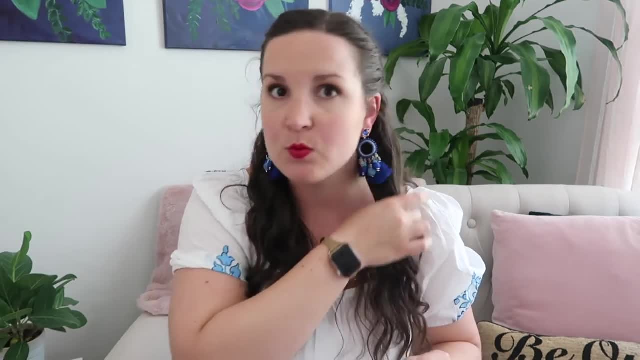 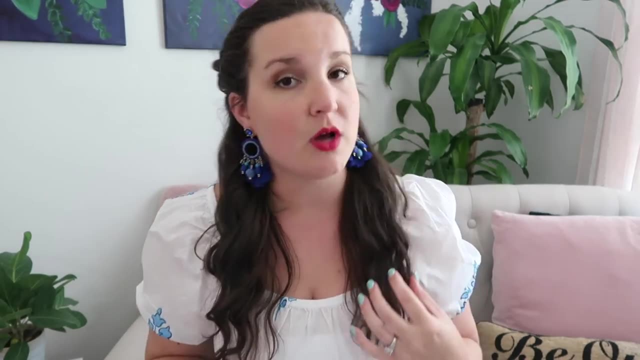 a year or two of each other that have like a texting group And anytime we have a question we're like: Hey, how did you do this? Hey, did you hear that? Like we all cause we happen to work, you know similar. If you do not work near people that you went to college with. 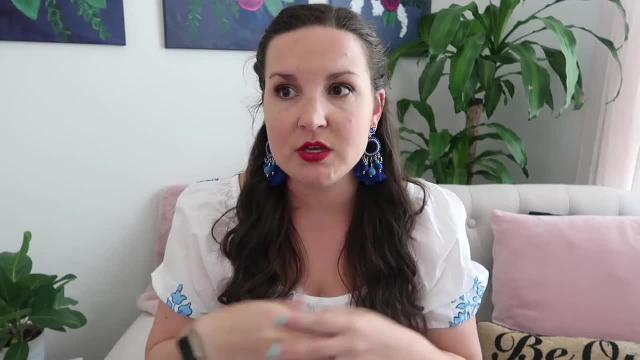 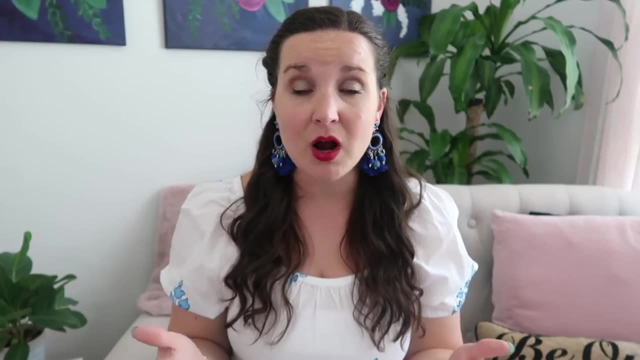 then you can reach out virtually. You can also reach out to the other schools, like literally go online to the other schools and figure out who their music teachers are and send them an email because they're probably going to want to like get together, If, like seriously, if the teacher 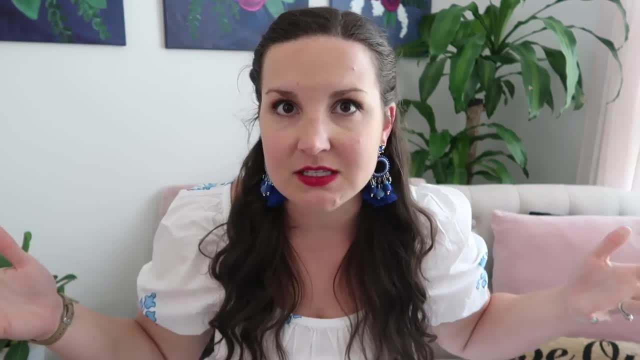 down the street from me, emailed me and was like: Hey, I'm going to do this, I'm going to do this Like some help. I'd be like: yes, please, Let's talk, Let's go get coffee, Let's you know. 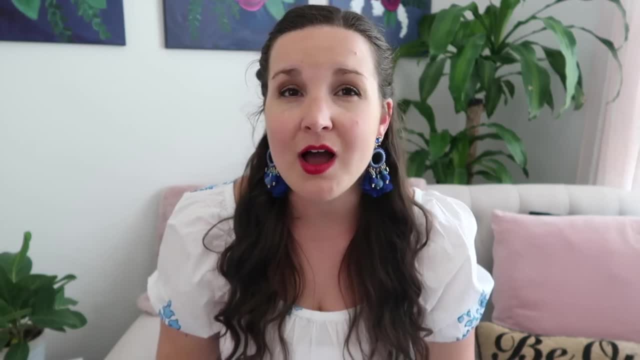 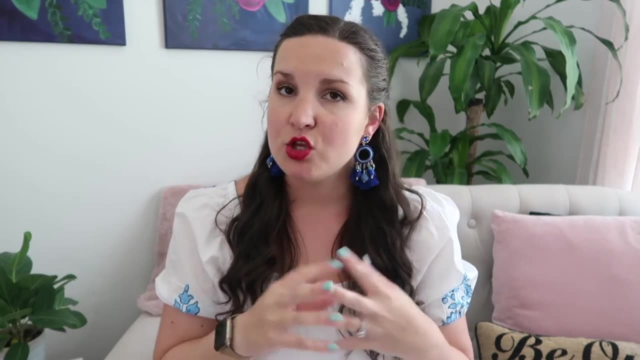 discuss let's you know text And I like not all teachers are willing to help, but a lot of teachers are And just having those people is going to make a huge difference. If you're in a bigger district, then you might even have, like music teacher mixers or like different things, like 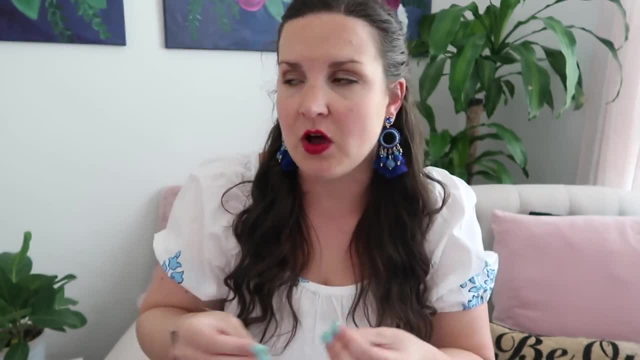 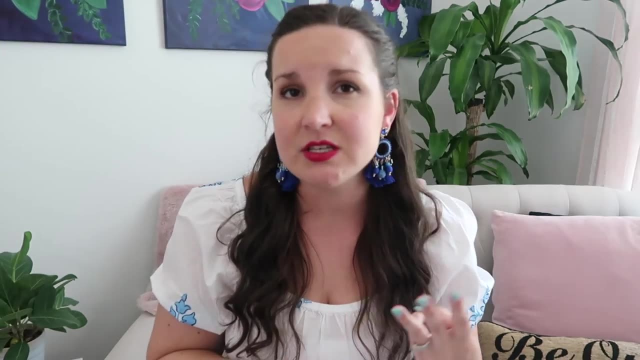 that in meetings, Make sure you talk to people, make sure you go first of all and then make sure you talk to people doing other things, Like if you're doing honor choir, if you do band, if you like, those things are also going to help you. 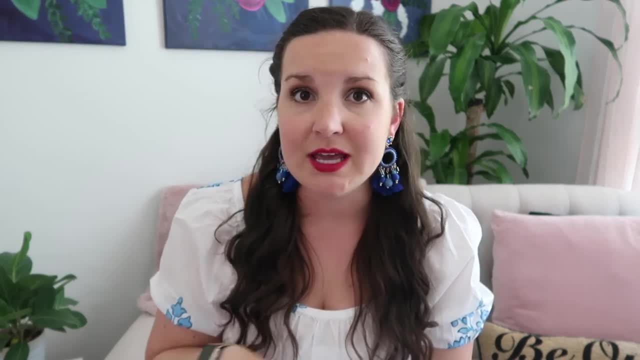 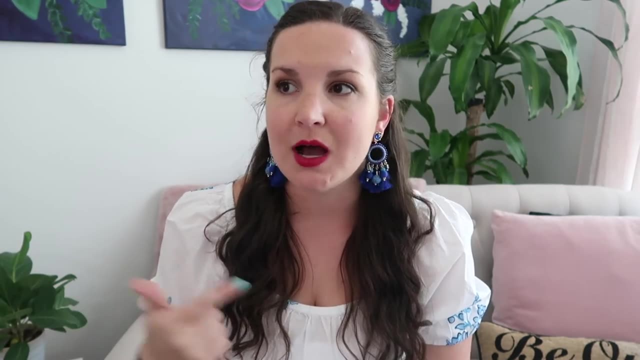 Like connect with other music teachers. You can also like take a course or take like a level- So like a Kodai level or an ORF level- and that's going to connect you with a whole bunch of people who not only are teaching elementary music but are also the kind of people who are willing to 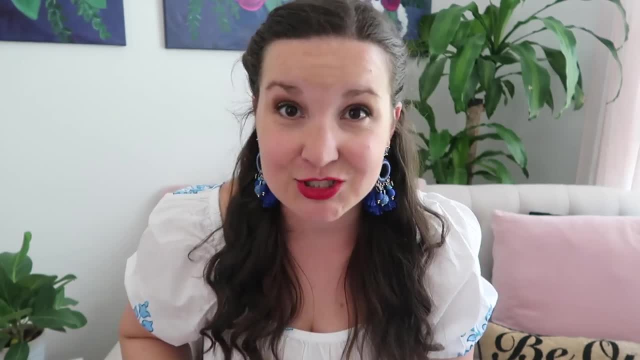 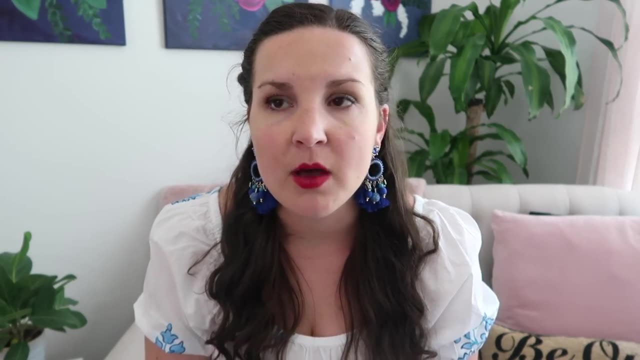 give up time to learn more, to be a better teacher, which is the kind of teachers you want to be friends with, So that will help you connect with people as well. And when all else fails, find people on Instagram, go like we. we live in the age of technology. We live in the age of technology. 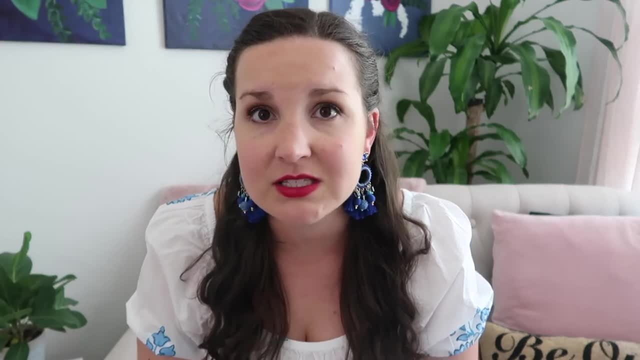 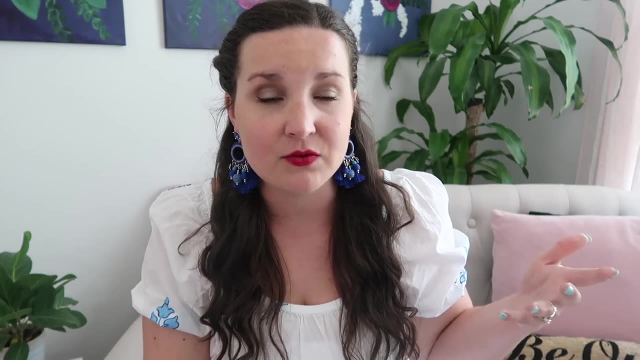 I have, literally, you know, I have friends who are teachers that live in different states and we like FaceTime and I've never met them in person, but we meet online, which, you know, it's like, definitely, things that our parents told us not to do when we were kids, but times have changed. a 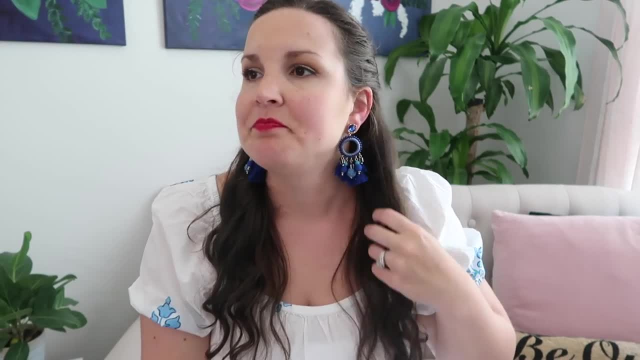 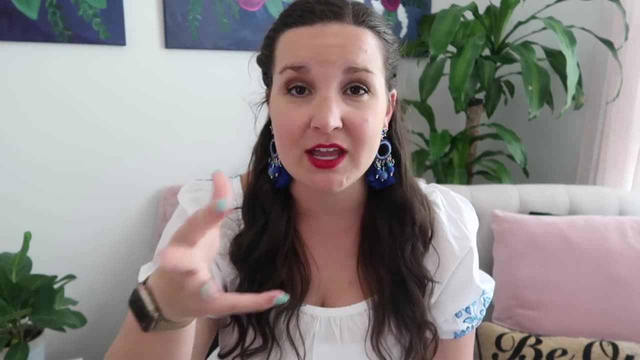 little bit and, you know, be smart about it, Don't be an idiot. but still, you know, find people on Instagram, find people on Facebook, join the Facebook groups. but even just like consuming videos that I create because I talk about elementary music stuff is going to help. 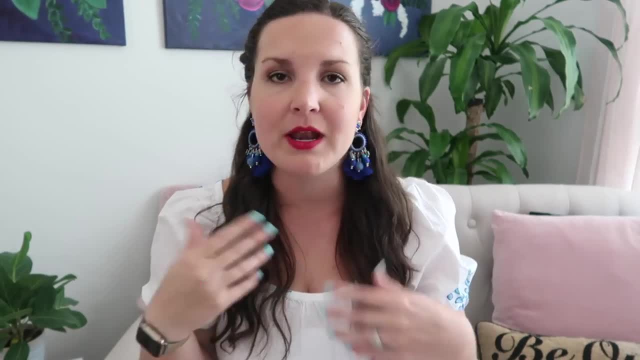 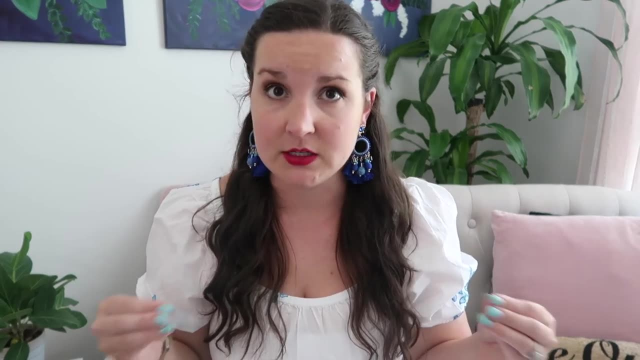 It's not the same. It's not the same as connecting with people, but it does help a little bit to get at least a little bit of ideas and be on the same page If you're like, really lonely, if you're really, you know, isolated. but find a person in person, if at all possible, who also teaches. 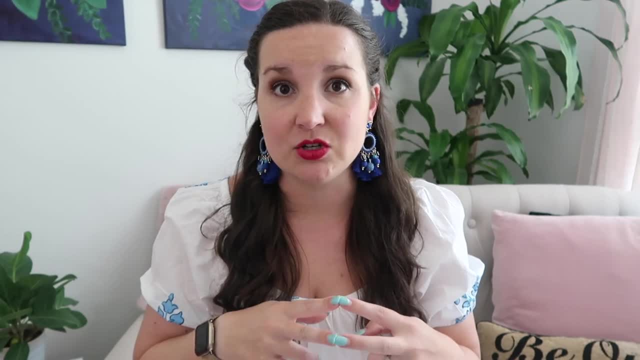 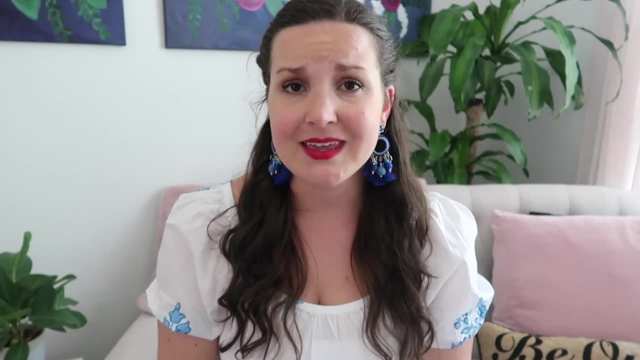 elementary music and connect with them as much as you can, because you're going to need a buddy, You're going to need someone that you can text and be like yo, I don't know where this stuff is, What do we do? And if they're in your district, even better, because 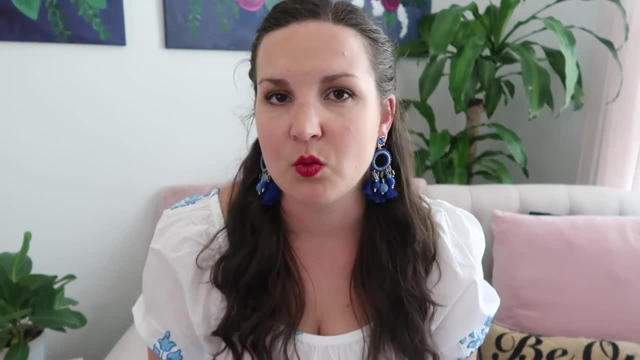 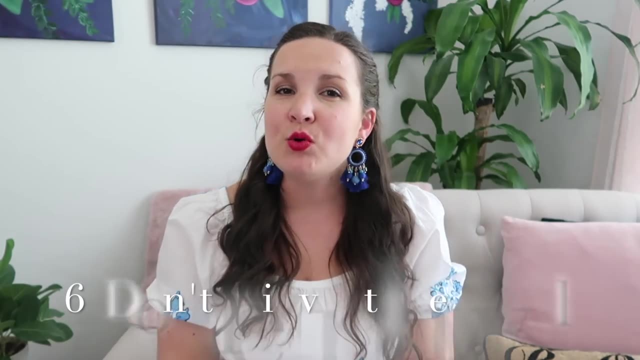 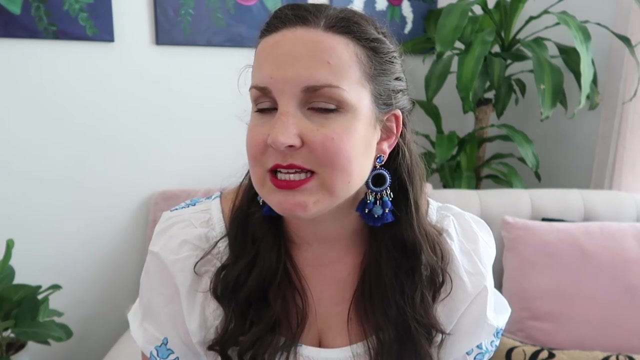 sometimes districts do things that you're like: what, what is happening? So that's helpful too. Number six is: don't reinvent the wheel. It can feel very exhausting your first year of teaching because you just don't have very many lessons, because you haven't done. 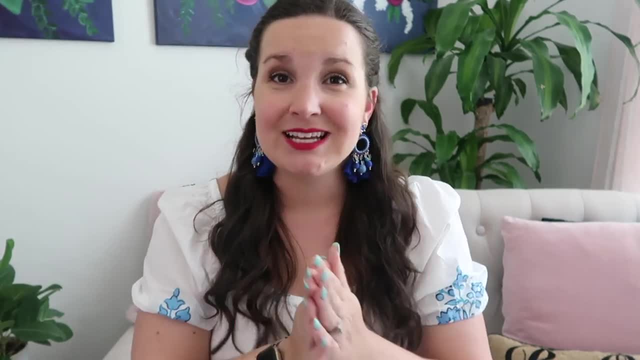 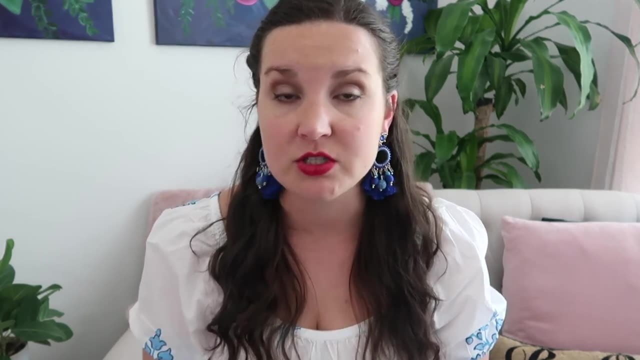 anything. So good news is: next year you'll have a whole year's worth of lessons that you can go back on, But this year you're going to feel like you just have so many things you have to come up with yourself. You don't have to do a lot of things, So don't reinvent the wheel. 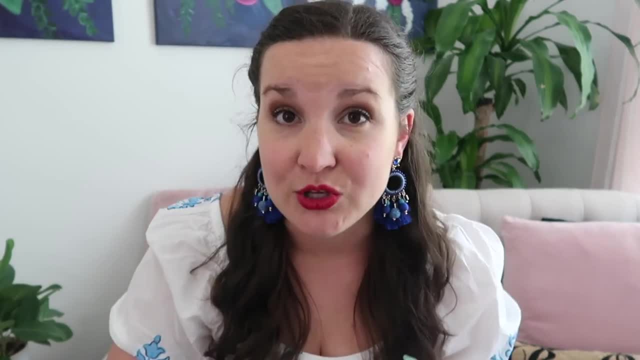 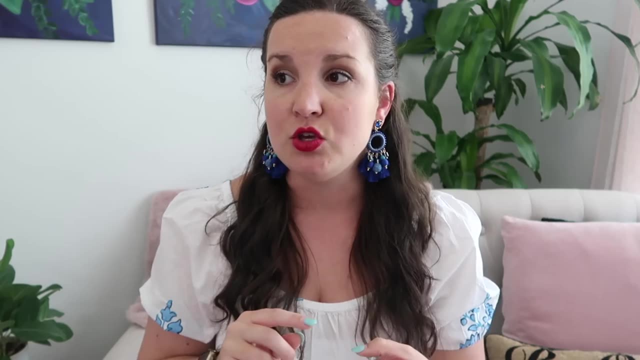 You don't have to come up with them yourself. You are welcome to use things from the internet. Seriously, I have like a bajillion different videos you can watch for lots and lots and lots of different ideas for lessons. You can buy things off teachers, pay teachers, You can connect with. 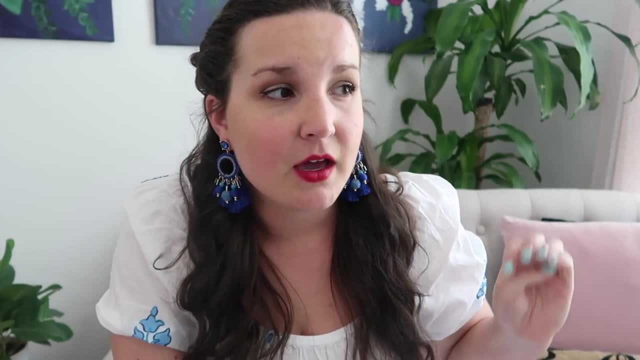 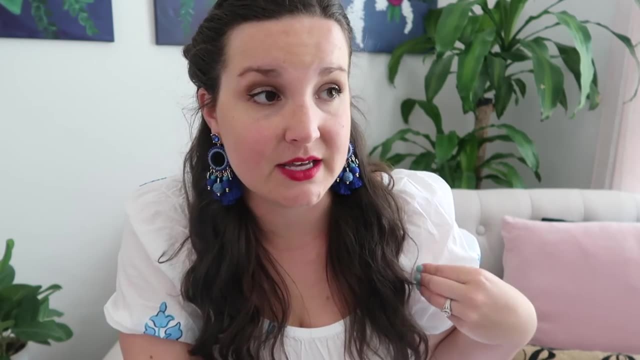 that teacher down the road and ask them what they're doing. You can even combine lessons So you're not writing six different lesson plans. Yes, friends, that is okay, Or at least I say it's okay. Maybe your district doesn't say it's okay, but I say it's okay. So what I mean by that is: 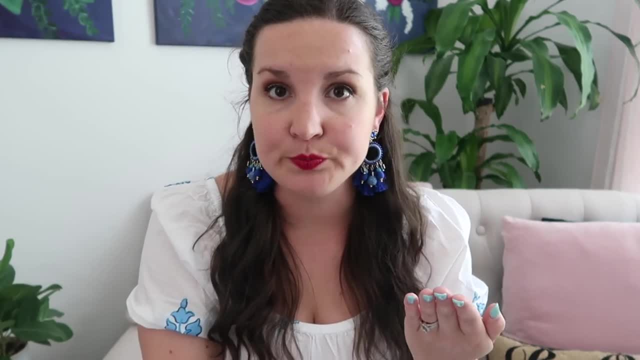 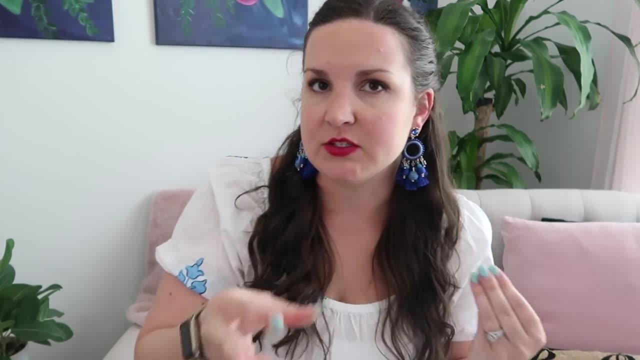 when I first started, I had a lesson for K through two and a lesson for three through five, Okay, And we switched them up a little bit, Like obviously I'm not using the same terminology with kindergarten as I am with second grade. Like we changed a little bit of things, but overall we 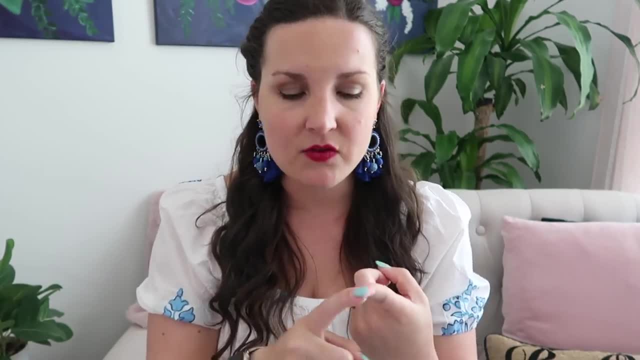 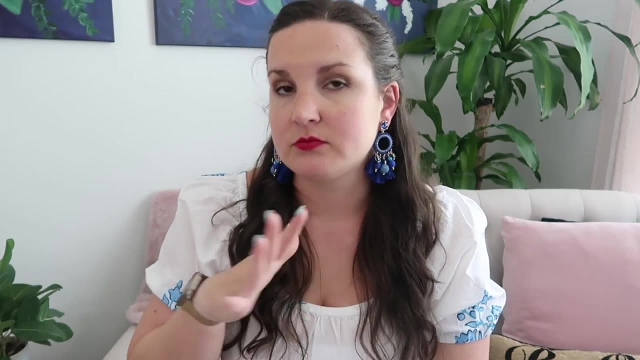 were doing the same type of things And that way I have less to remember And I also have less to plan, because I just have no idea what to do. Now, after I got through that, year felt pretty good. Year two I did K one, two, three, four, five. 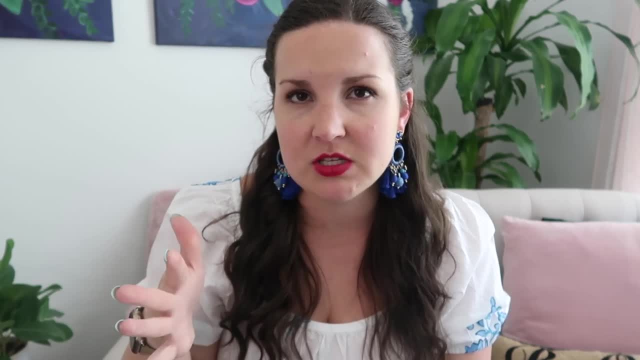 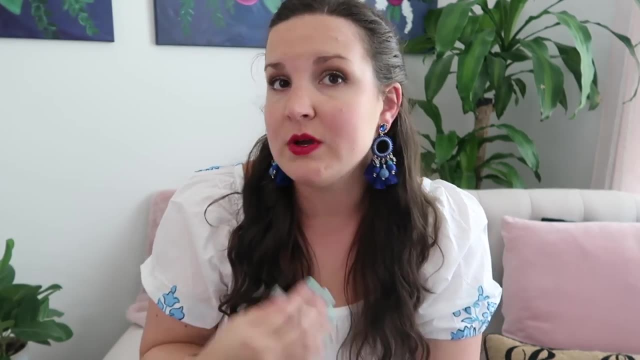 We're at the point where pretty much everyone gets their own lesson Most of the time. sometimes I combine four and five, Sometimes I do combine first and second. I don't teach kindergarten anymore, Um, but overall we have mostly our own lessons, because I'm now years. 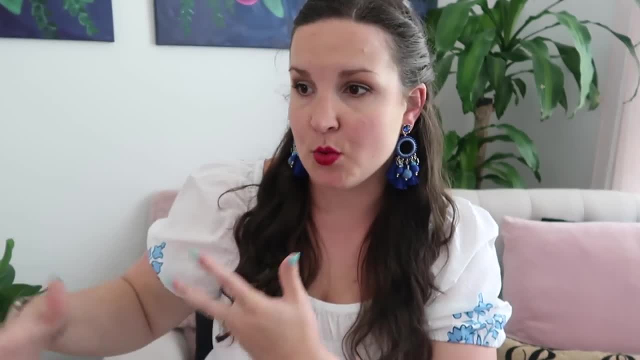 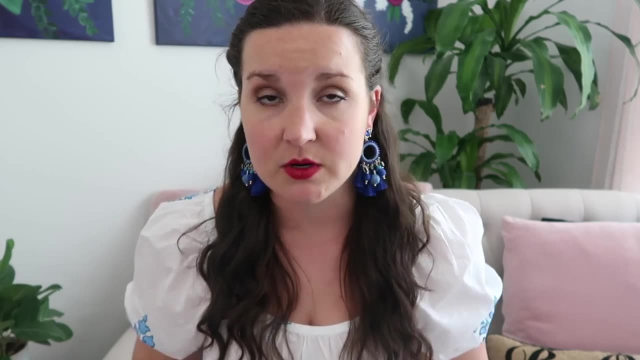 down the road and I have a buildup, a library, a repertoire of different lessons that we can do, And I have like ideas And so adding something new is not as stressful. but if you are starting out seriously, do K through two, three through five and go for it, And it will be. 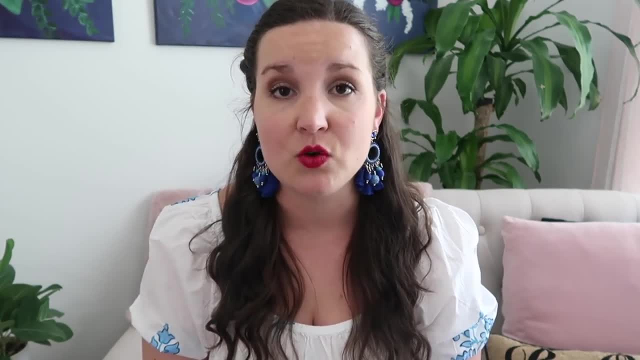 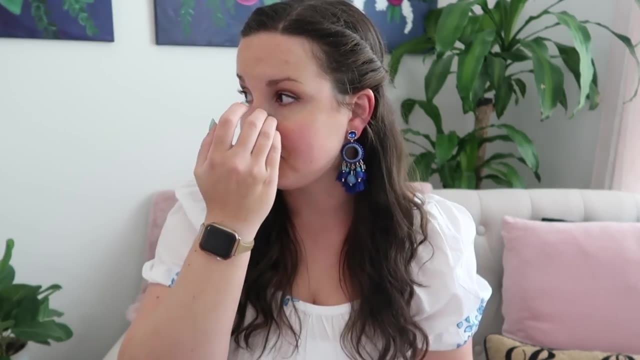 be fine. Um, don't stress too much about it. You do not have to reinvent the wheel, and you're welcome to steal things from other people too. I mean, steal them legally, Don't you know, copyright infringed. but yeah, Yeah, This was my last actual tip. And then I have a. 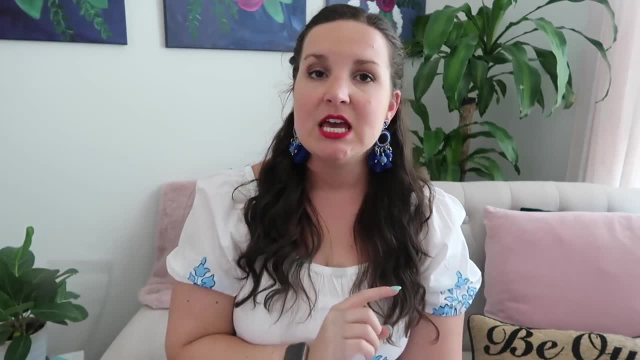 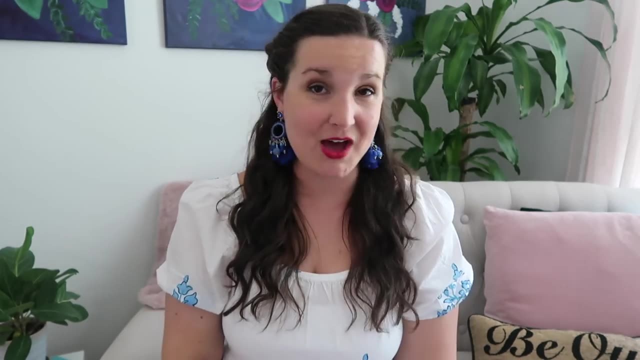 couple of things that are really important for you to remember. So the tip number seven is: keep learning. learn as much as you can, because, again, you didn't learn everything that you could have in college, because it's just not set up in a way that is conducive to all of that. 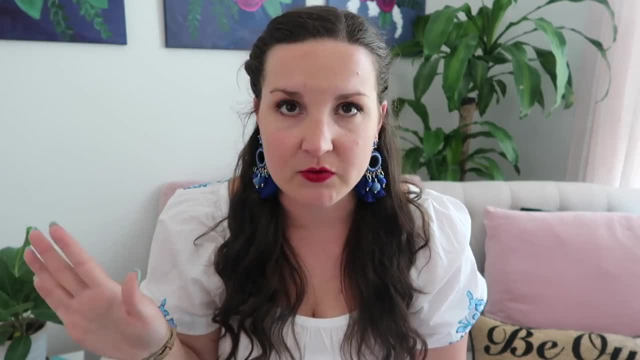 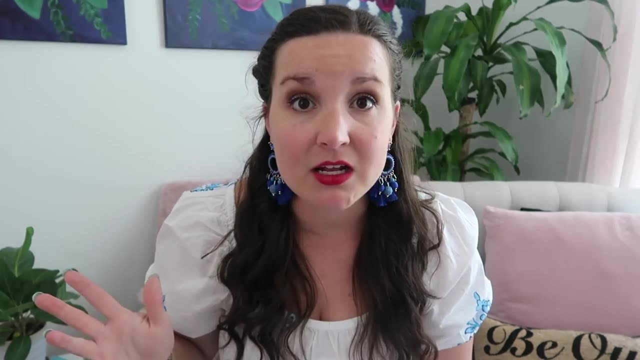 Because you have to take all of these different classes. Um, that's a topic for another day, but my point is keep learning. watch people on YouTube, get some music teacher podcasts, get some books, take a Kodai level, take an ORF level, take some classes like, whatever it is. 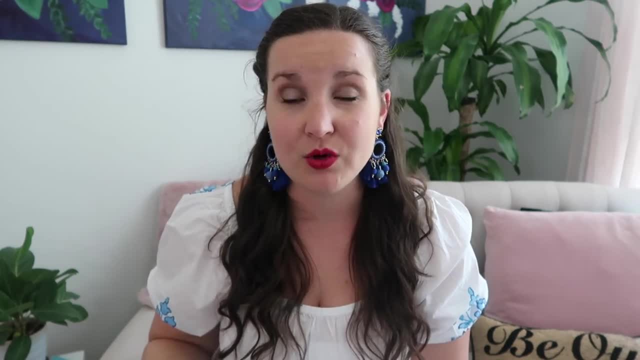 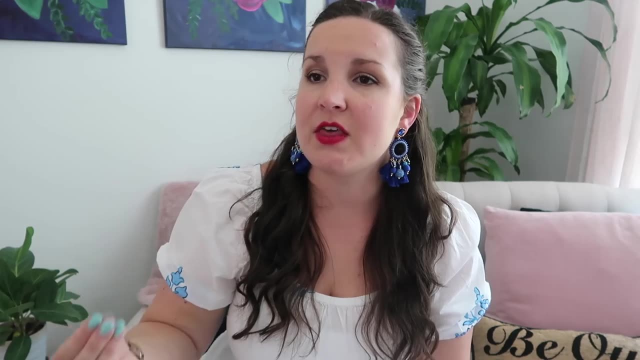 that you can do. do the things that are going to help you learn more, because the more you can learn, the better you will be And the better you teacher you will be And also less stressed you will be, because you will have ideas and you will have things and you'll know what to do instead of 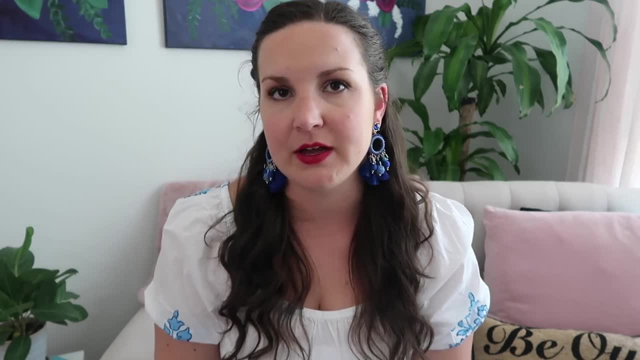 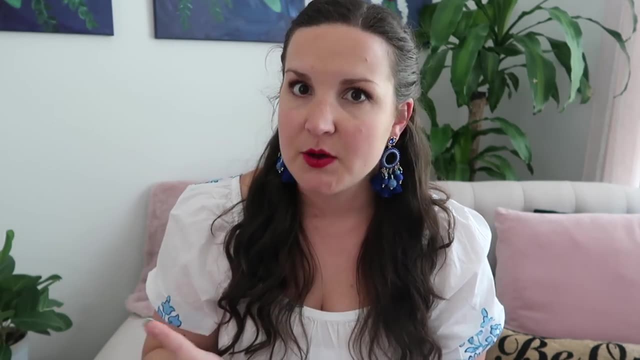 being super, super, super lost. You're going to be lost either way, But if you keep learning you'll be a little bit less lost. All right Now a couple of things that music teachers need to remember when they're starting out is number one. it's supposed to. 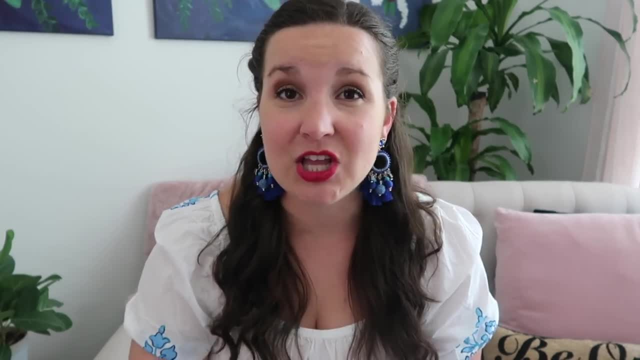 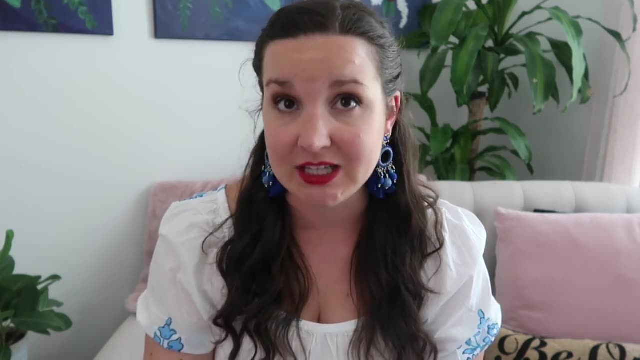 be hard. If it feels hard, it's because it is hard. It's a lot, It's hard. You probably aren't prepared for it. That's okay, Do your best. It's not that you're doing it wrong, It just really is. 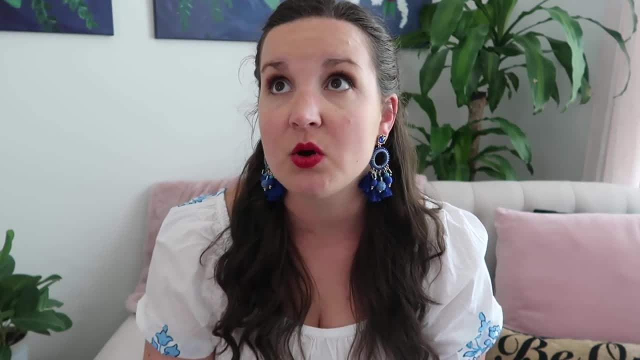 that difficult. So if you get halfway through your year and you're like, Oh my gosh, this is so hard, Why is it so hard? It's hard because it's supposed to be hard and it will get easier. So don't stress about it, You're not doing it wrong. 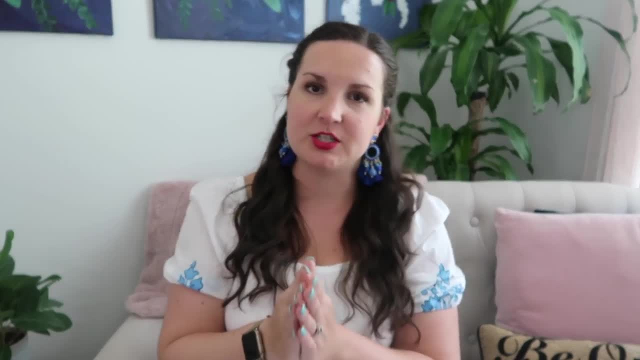 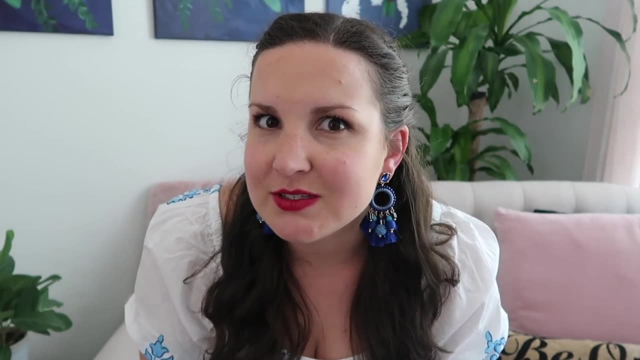 Just go for it. The other thing I want you to remember, as you're going through especially your first year of teaching, is that it's okay to have fun. Seriously, Teaching is fun, and especially teaching music. Like you could have been, you could have become a calculus. 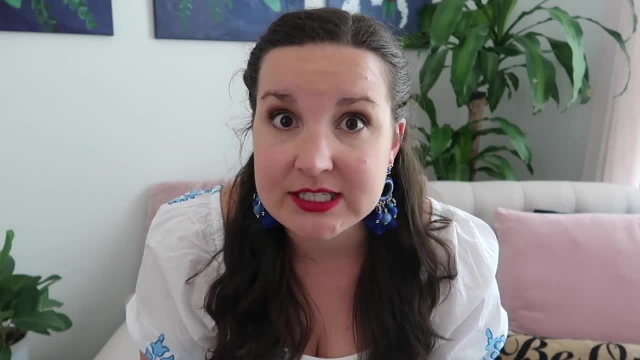 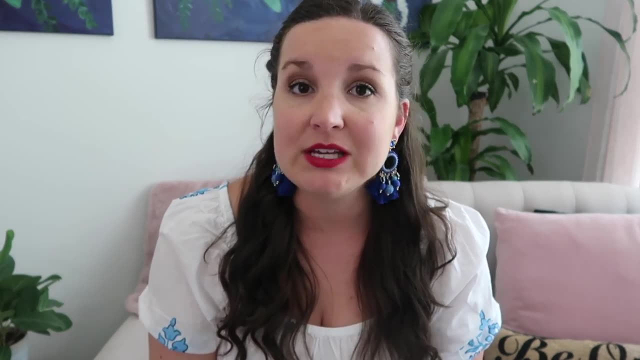 teacher and instead you're teaching little kids how to sing and play games Like it's great. It's not always fun, but make sure that you enjoy the fun parts and really try to like enjoy that. When I'm playing a game with the kids, I try to like be in the moment. 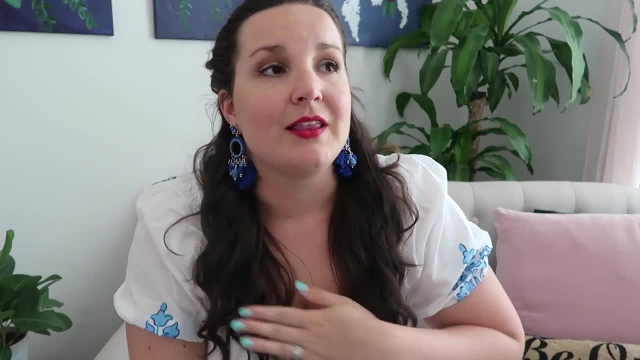 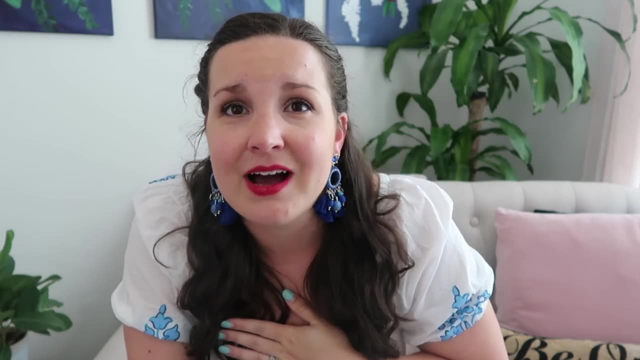 and really enjoy it. when you get like, Oh my gosh, when you get like a whole kindergarten class and they're like all singing in tune and they're cute little voices, And Oh my gosh, it just warms your heart Like. enjoy those moments, because it's not all fun and it's not 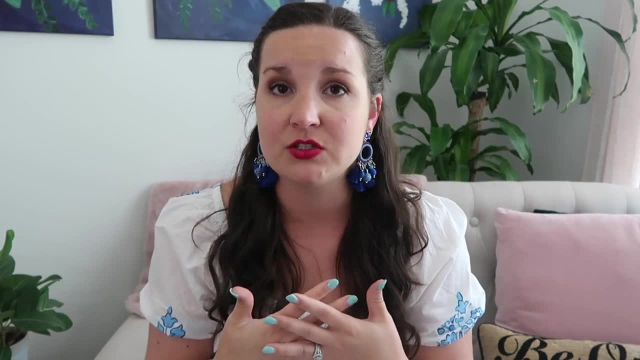 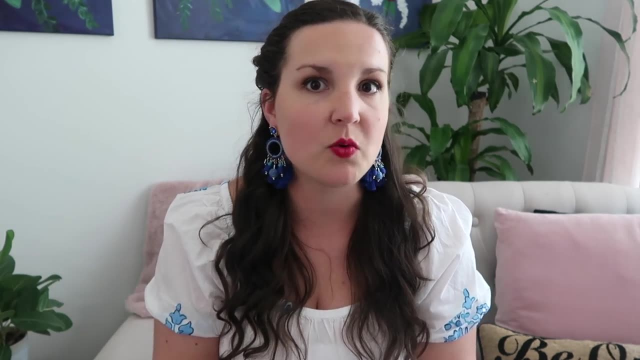 all sweet and it's not all cute. Make sure that you enjoy all of the good parts so that you have something to hold on to for the times when it's not so great, Like February. February is usually when everything is just like the world's going to end. 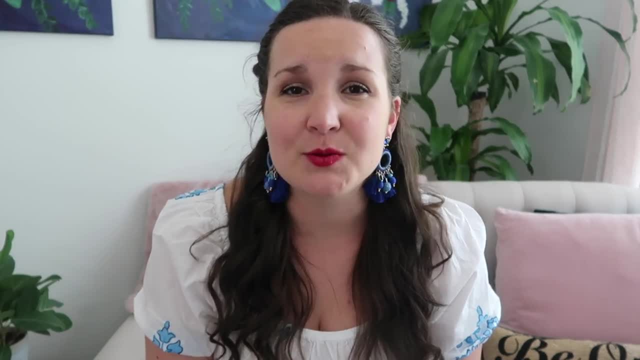 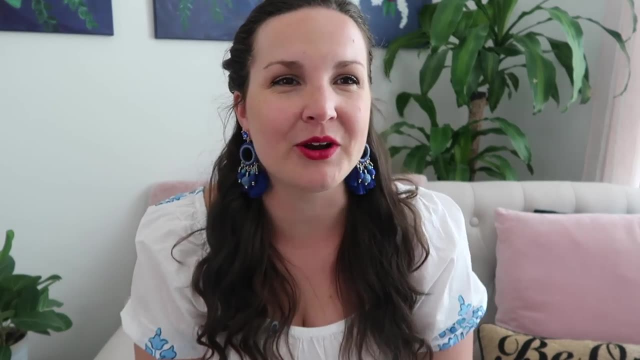 but it does get better, because then May comes. Make sure you enjoy it. I tell my husband all the time I'm like: look, some people go to work and they're bored. I am never bored, Like I am never bored, At least I'm not bored, I'm always entertained. Every day is different, Everything.